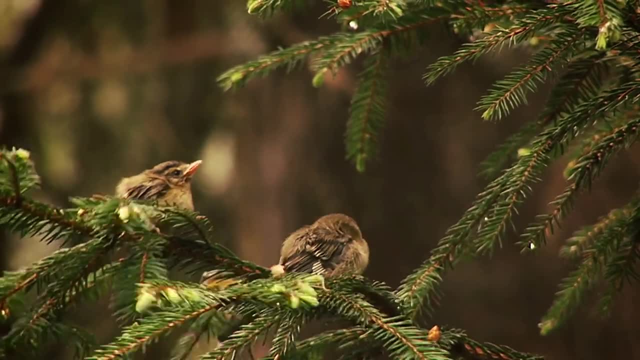 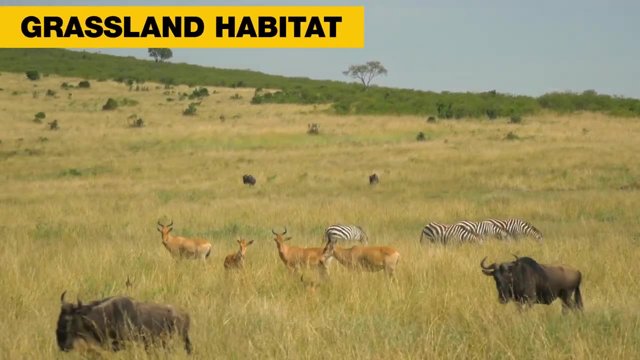 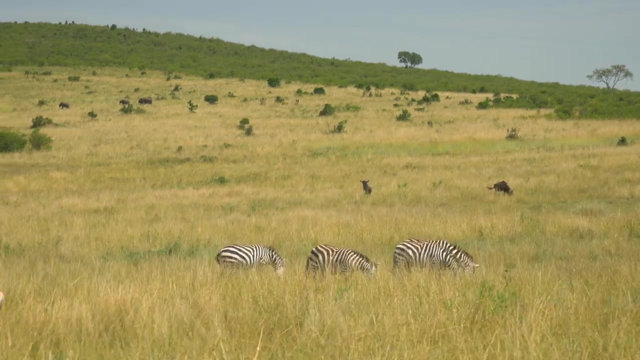 Let us learn the different habitats on our planet. Grassland habitat- Grassland biomes are found in warm, arid climates. They get just enough rainfall to support the growth of grasses, which are large plants that do not need as much water as trees. 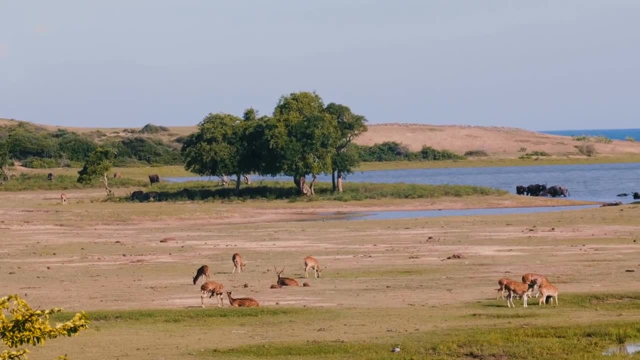 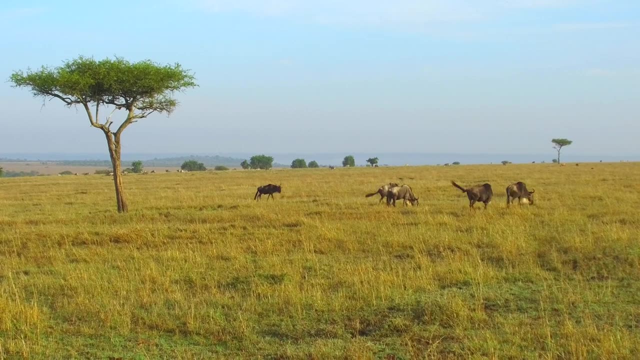 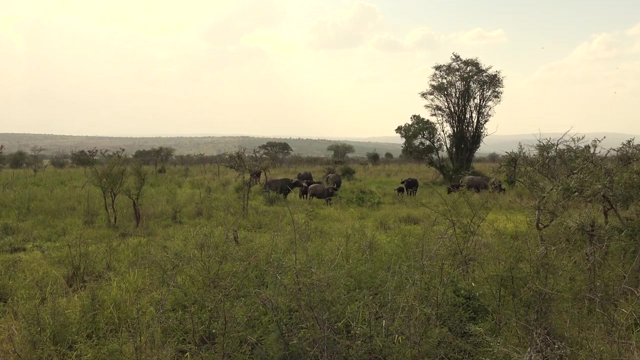 The plants that grow here range from tiny stems to tall grass-like stalks and small shrubs. The life in a grassland biome is also diverse. Many different animals and plants live there. Grasslands can be found in many parts of the world and in many different climates. 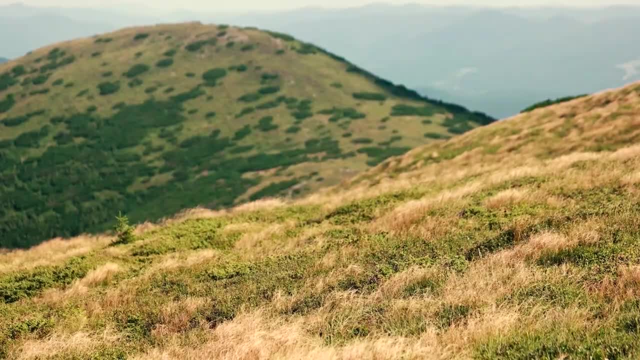 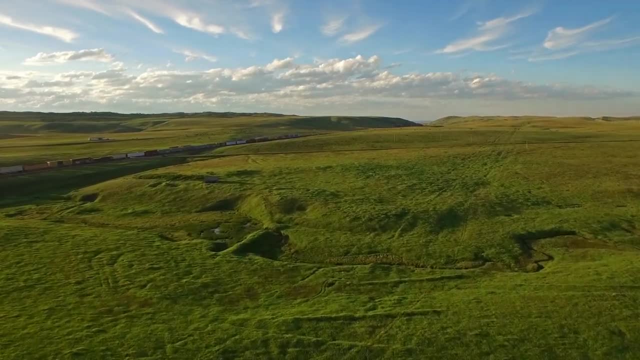 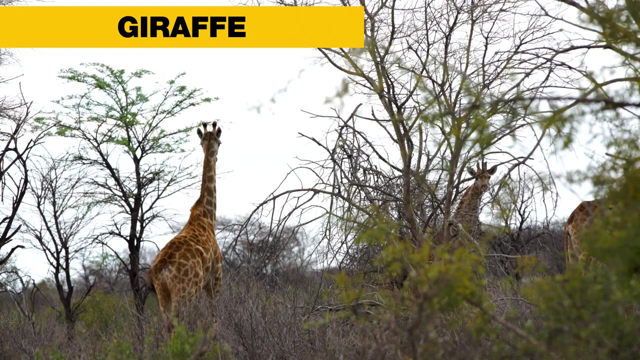 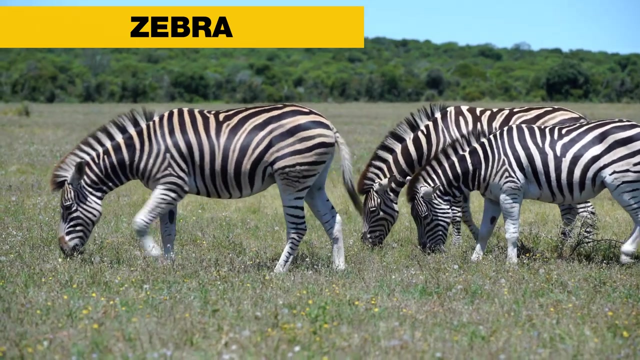 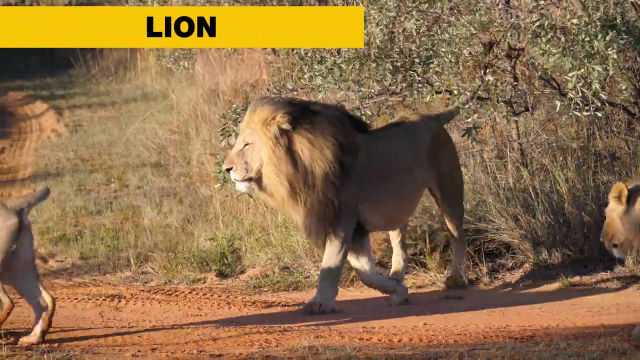 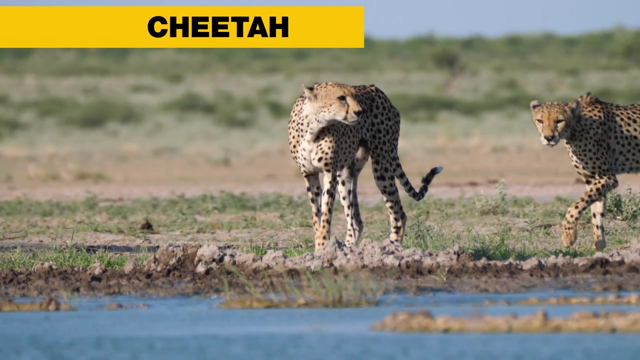 Grasslands are generally located between deserts and forests. Here are some animals that live in grasslands habitats: Giraffe Giraffe. Zikka. Howling Zebra. Howling Lion. Lion. Howling aval. Howling Lion. Howling Lion. Howling, Howling, Howling. 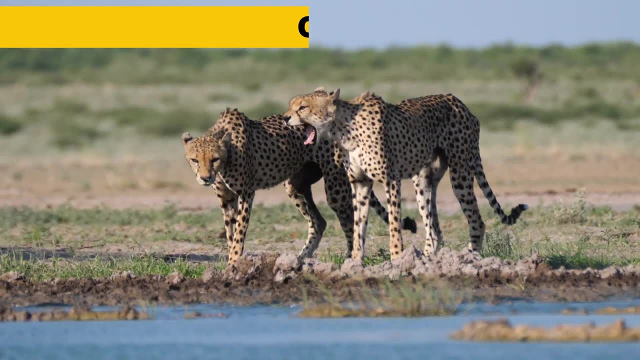 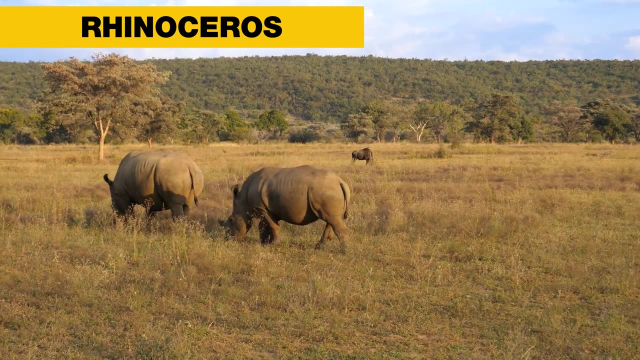 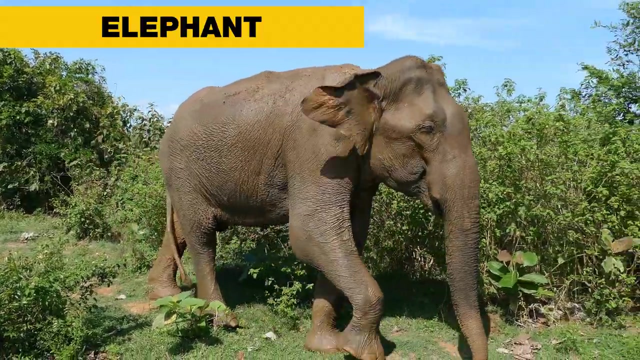 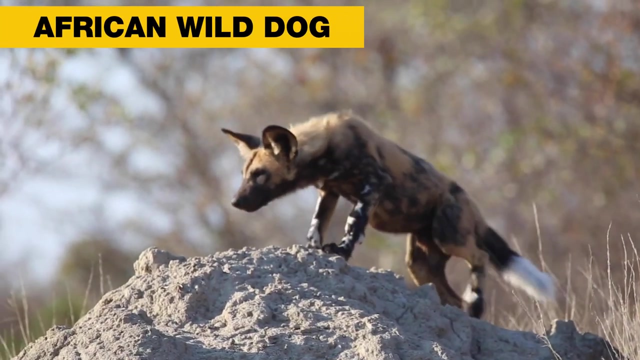 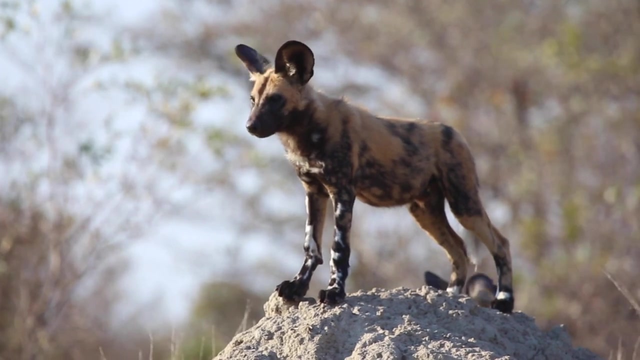 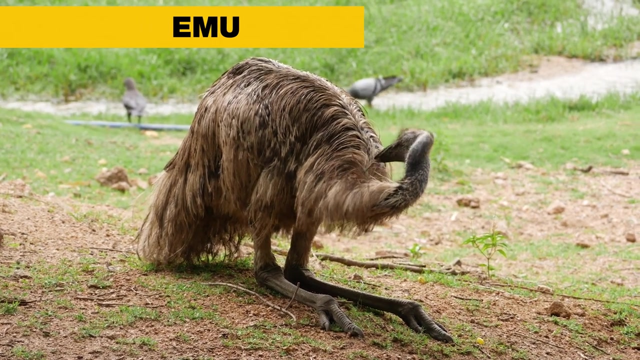 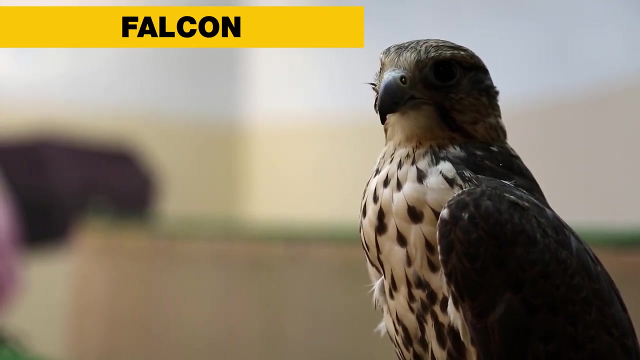 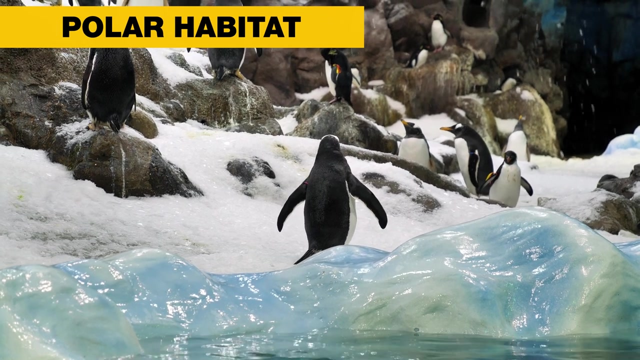 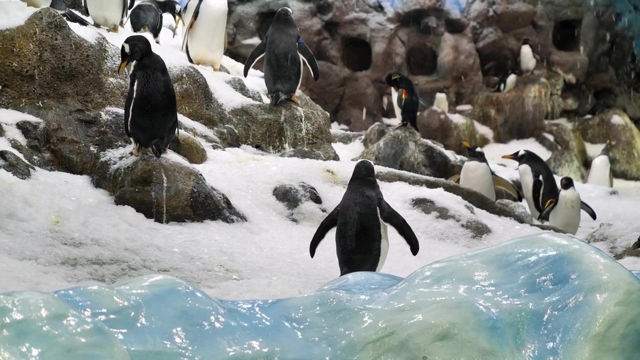 Howling, Howling, Rhinoceros, Elephant, African Wild Dog, Emu, Falcon. Polar Habitat. The polar regions are found at the top and bottom of the planet Earth. The north polar region is called the Arctic, and in the south, the polar region is the continent of Antarctica. 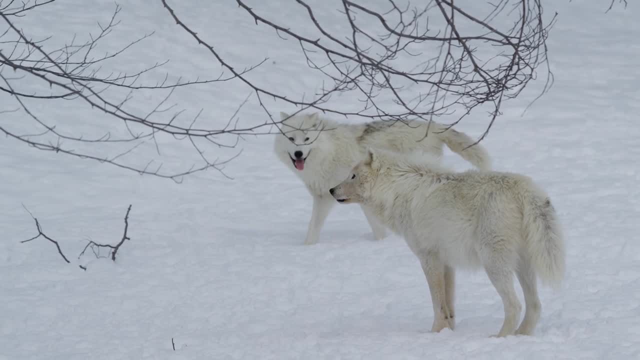 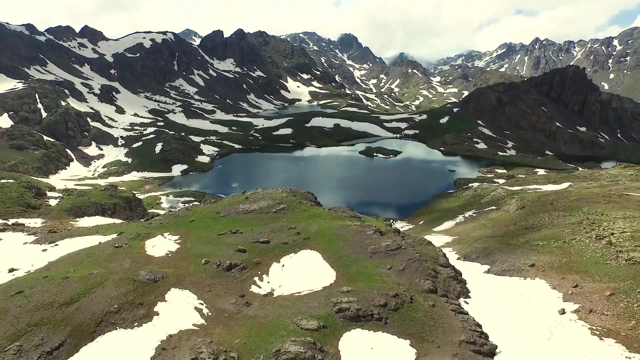 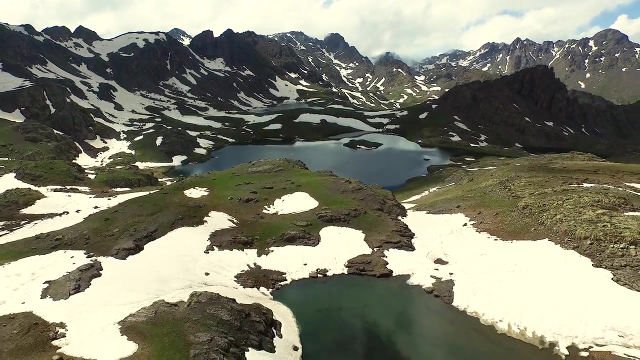 Both are characterized by their extremely cold climates, making them an important ecosystem with distinct physical characteristics, plant life and animals. Polar habitats have tundra, which is ground that is nearly always frozen. The very top of it will melt during summer months, so grasses and mosses can grow. 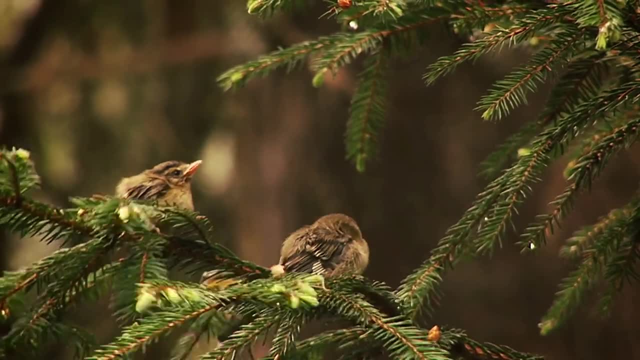 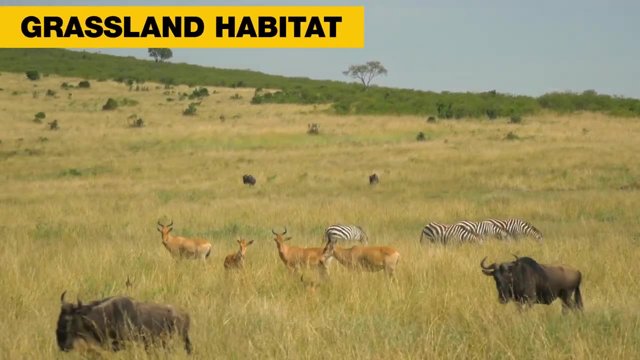 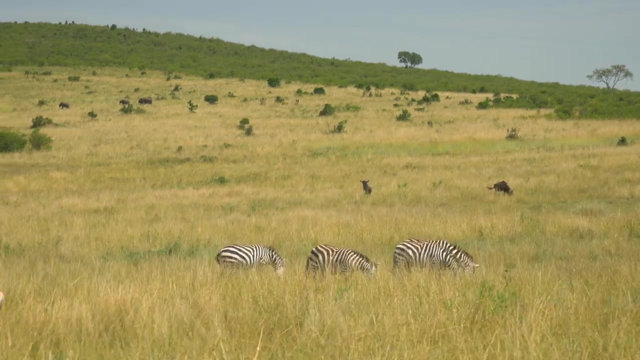 Let us learn the different habitats on our planet. Grassland habitat- Grassland biomes are found in warm, arid climates. They get just enough rainfall to support the growth of grasses, which are large plants that do not need as much water as trees. 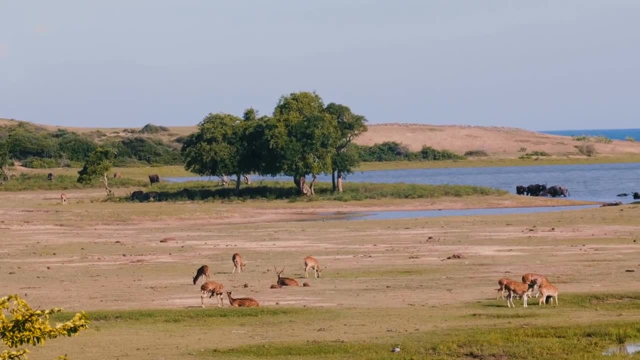 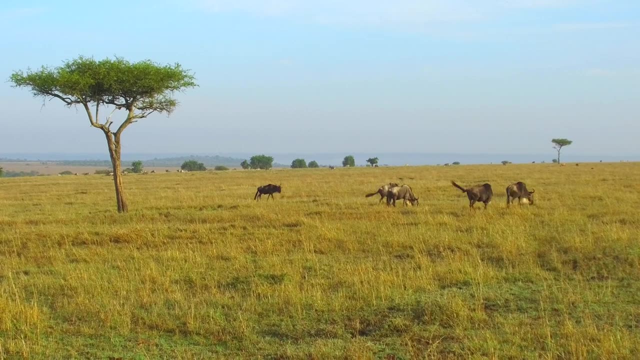 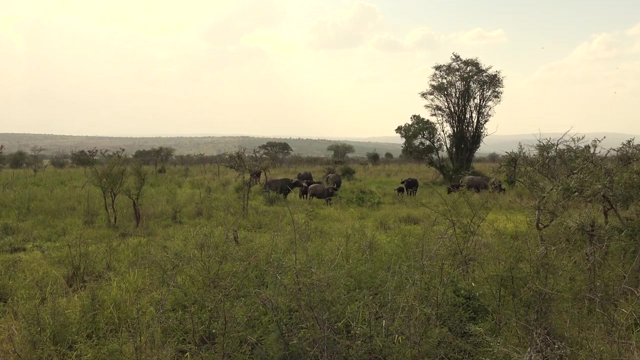 The plants that grow here range from tiny stems to tall grass-like stalks and small shrubs. The life in a grassland biome is also diverse. Many different animals and plants live there. Grasslands can be found in many parts of the world and in many different climates. Grasslands are generally located between deserts and forests. Here are some animals that live in grasslands habitats: Giraffe Giraffe Zebra Zebra, Zebra, Zebra Zebra Zebra. Lion, Lion, Lion, Cheetah, Cheetah, Chita, Rhinoceros. 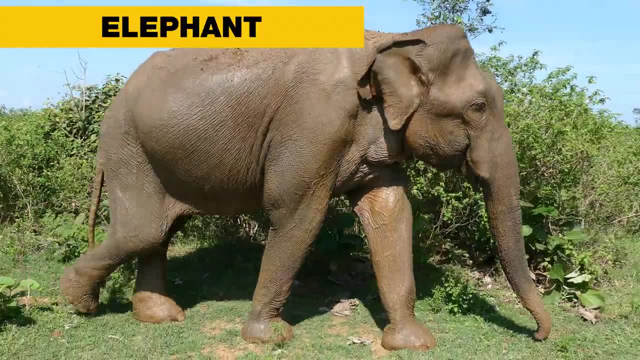 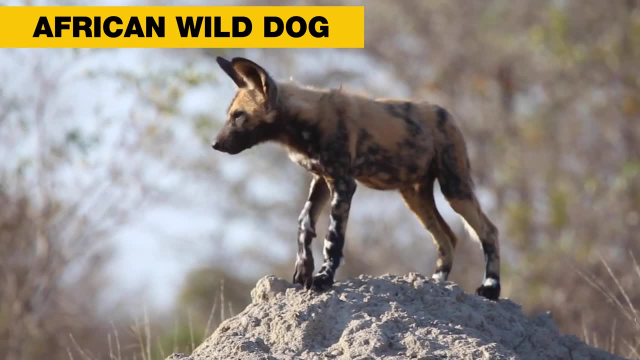 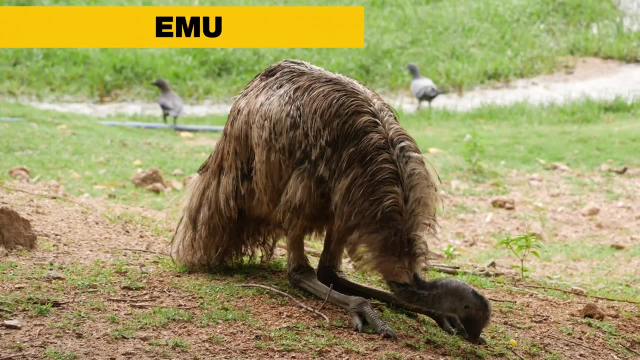 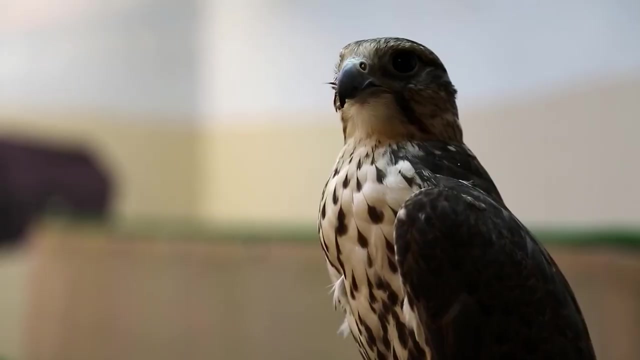 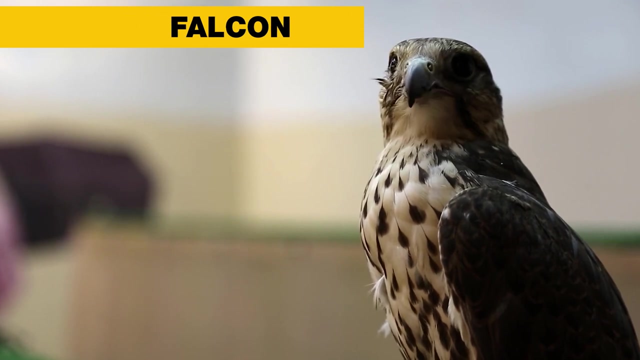 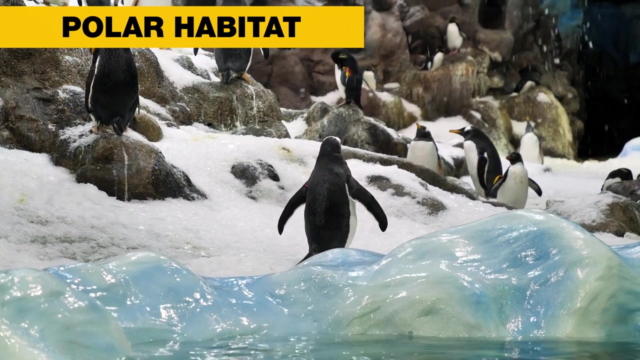 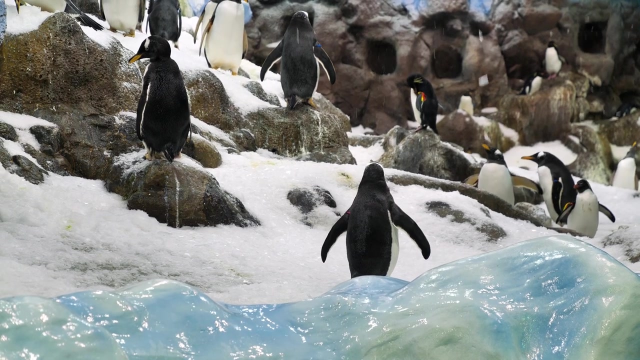 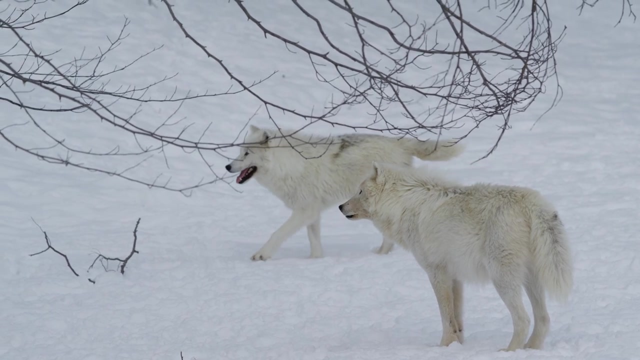 Elephant, African Wild Dog, Emu, Falcon, Polar Habitat. The polar regions are found at the top and bottom of the planet Earth. The north polar region is called the Arctic and in the south, the polar region is the continent of Antarctica. Both are characterized by their extremely cold climates, making them an important ecosystem with distinct physical characteristics, plant life and animals. 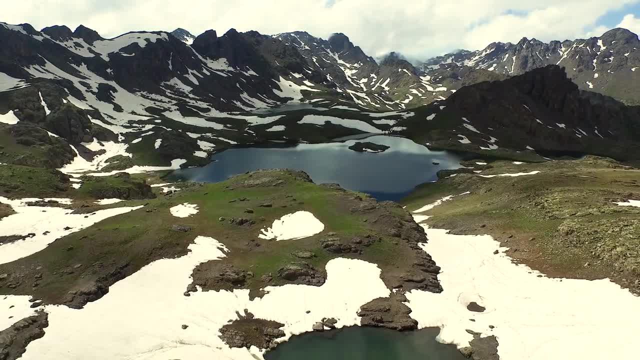 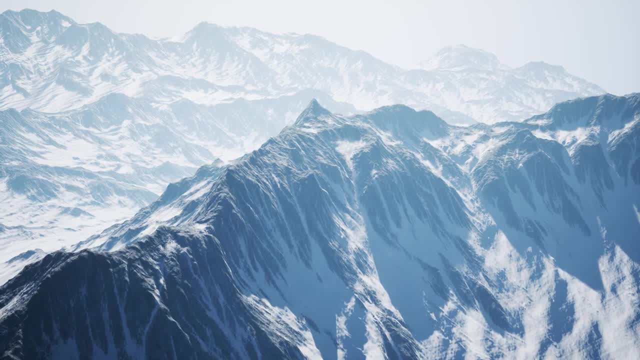 Polar habitats have tundra, which is ground that is nearly always frozen. The very top of it will melt during summer months, so grasses and mosses can grow. Animals are perfectly adapted to live in these regions. Here are some animals that live in polar habitats. 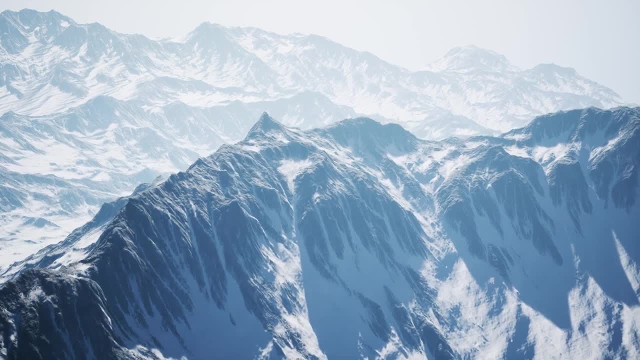 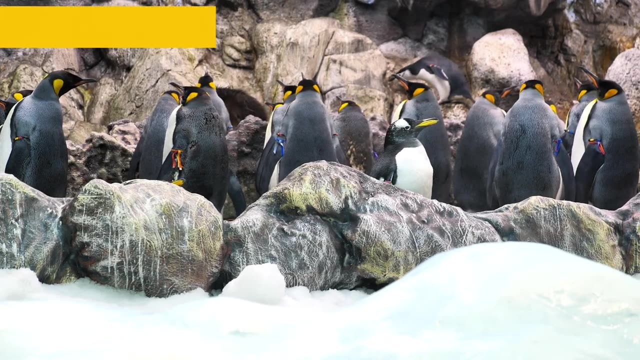 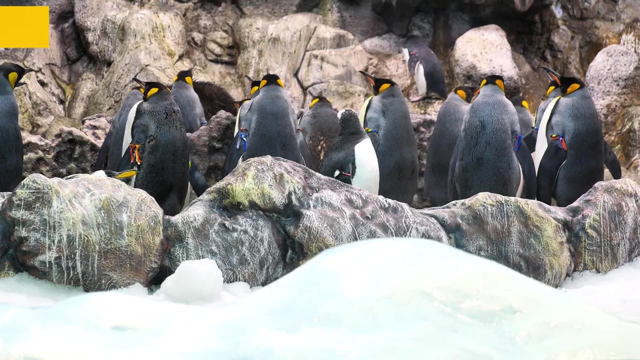 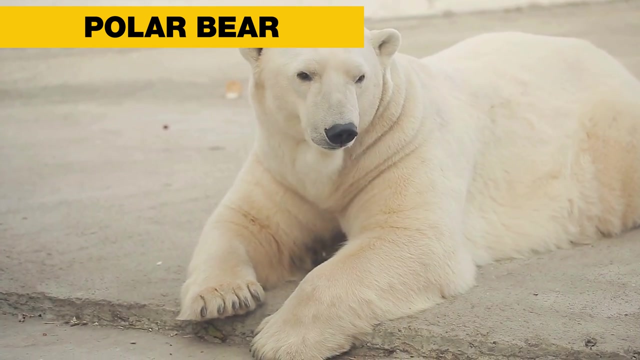 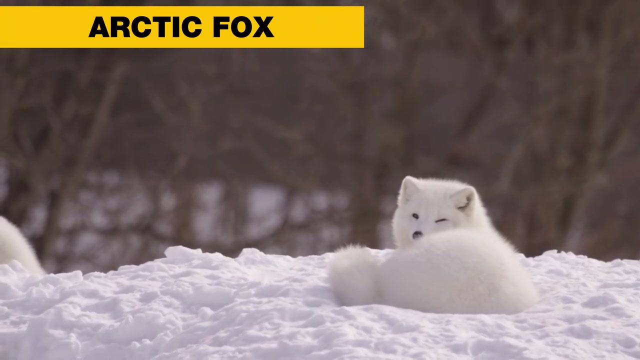 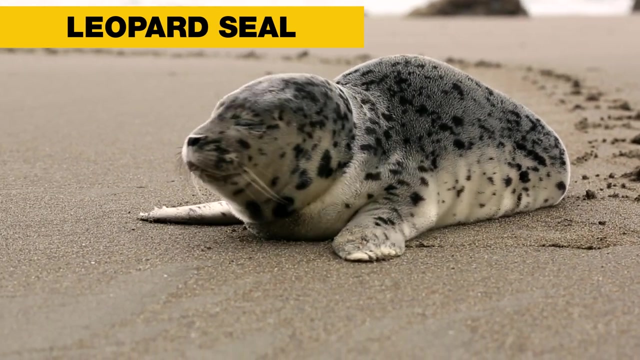 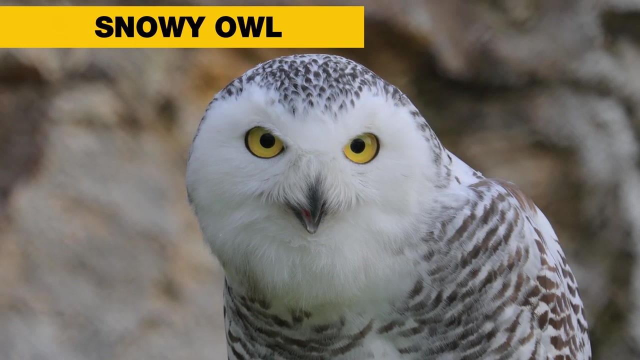 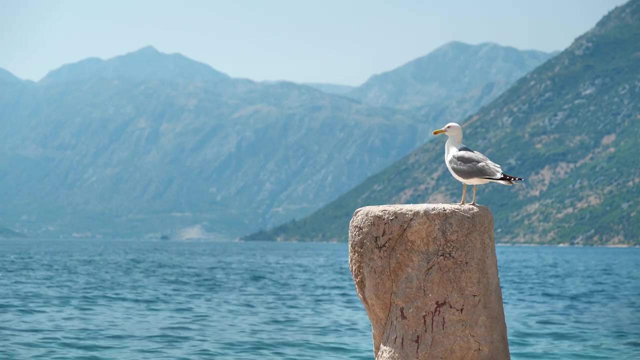 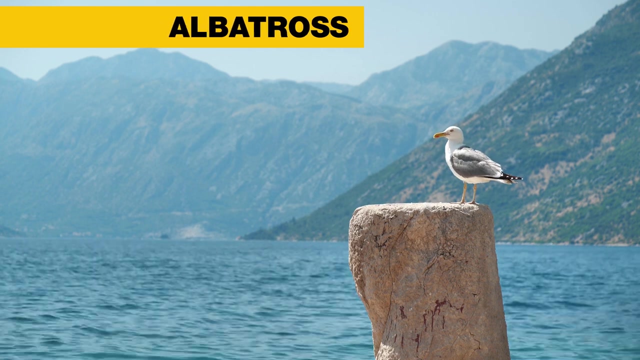 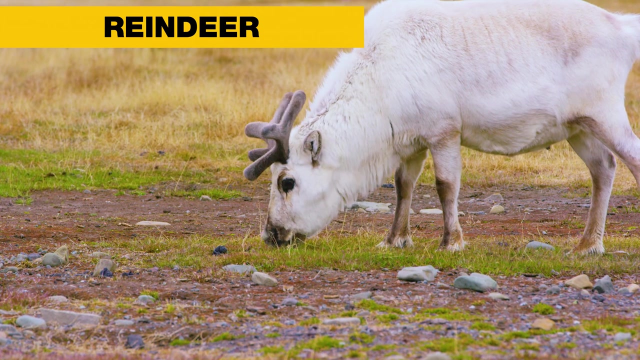 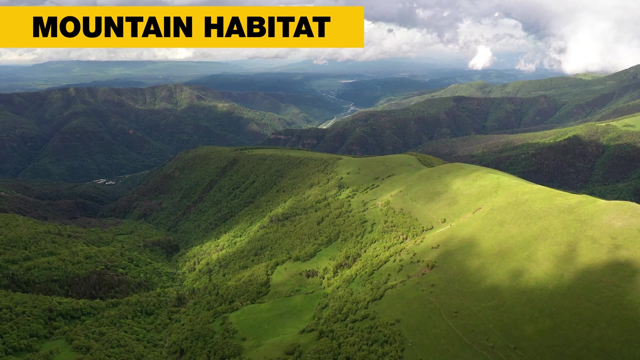 Animals are perfectly adapted to live in these regions. Here are some animals that live in polar habitats: Penguin, Polar Bear, Arctic Fox, Leopard, Seal, Snowy Owl, Albatross, Reindeer, Reindeer Mountain, Habitat Mountain. Habitat Mountains are home to plants and animals that are adapted to the very harsh weather conditions they experience. 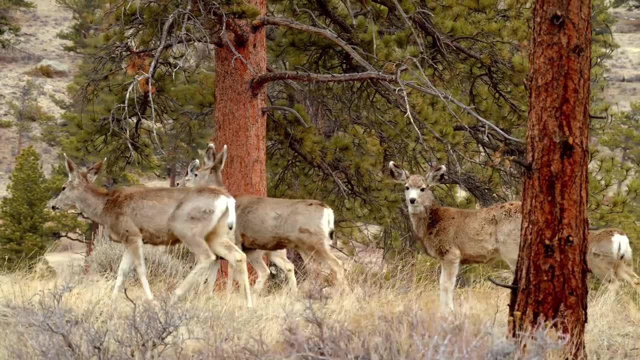 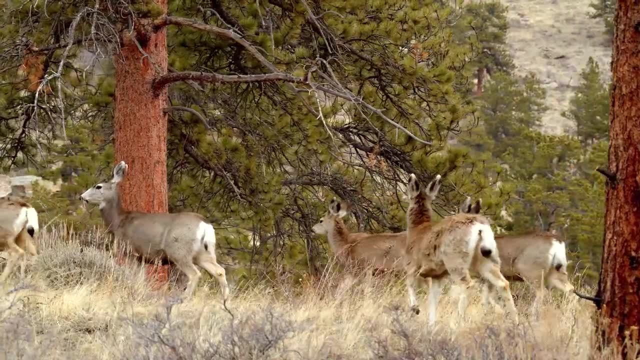 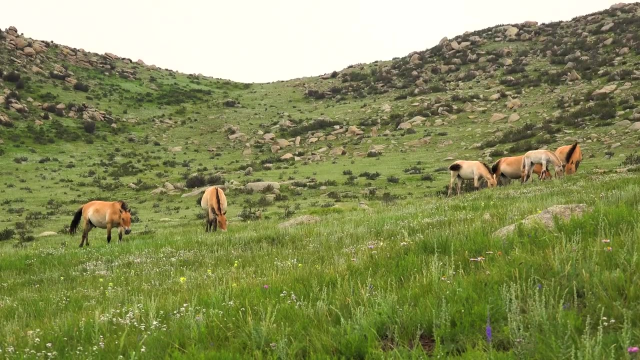 Most of the time it is cold and windy. The lower slopes of a mountain ecosystem are usually covered with forests, But as you go higher in the mountains, the air gets thinner, colder and less oxygen is available. Some plants do not survive at high altitudes because they require warm temperatures to grow. 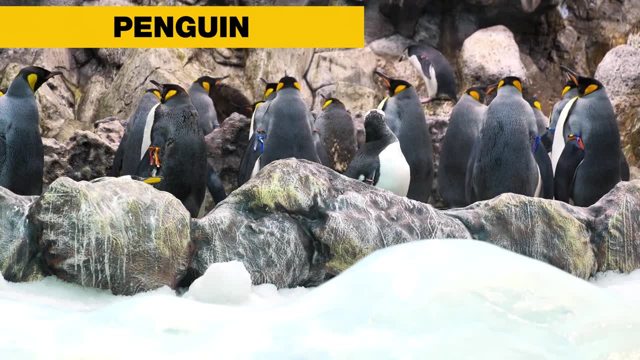 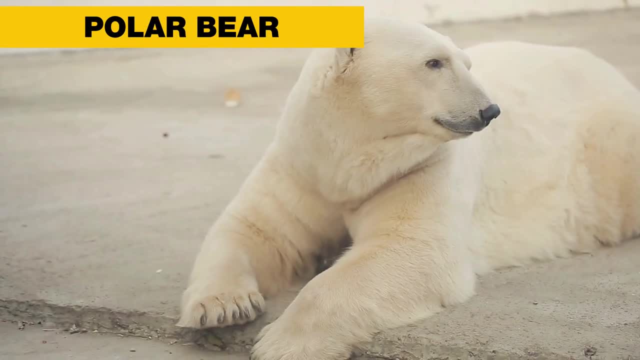 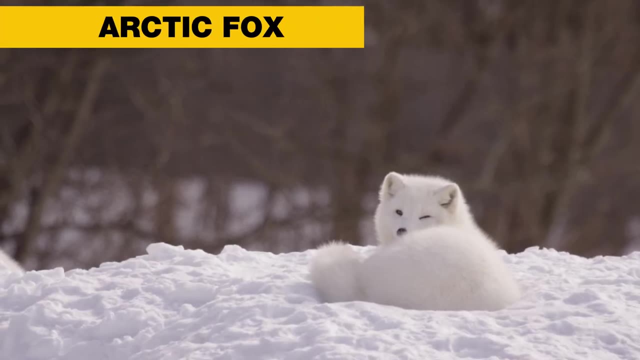 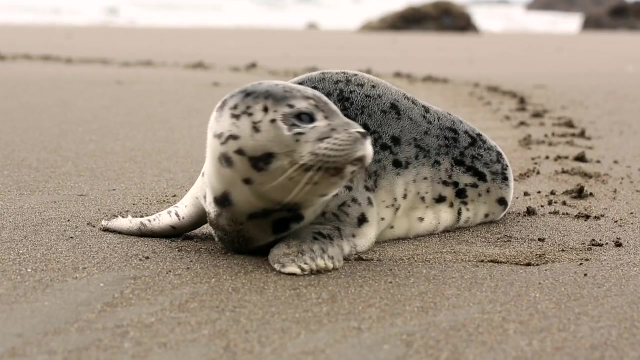 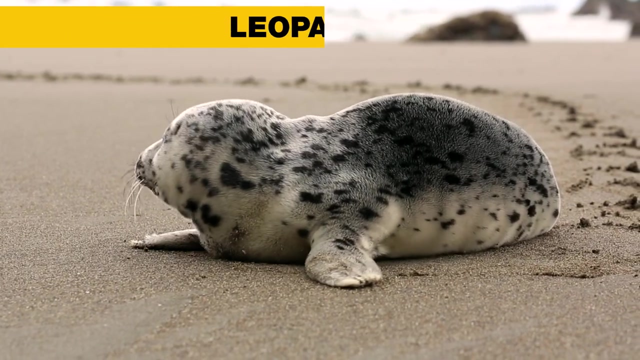 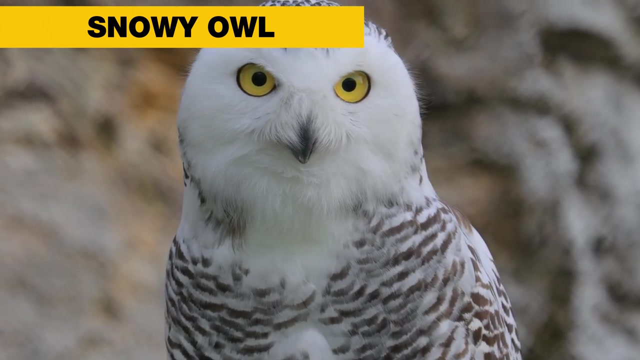 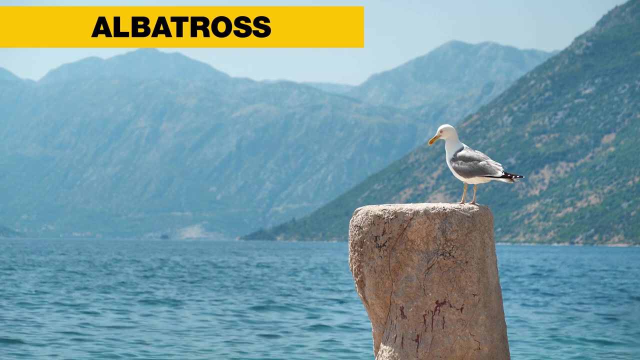 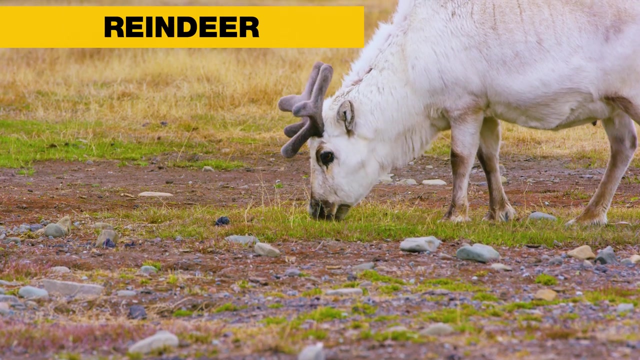 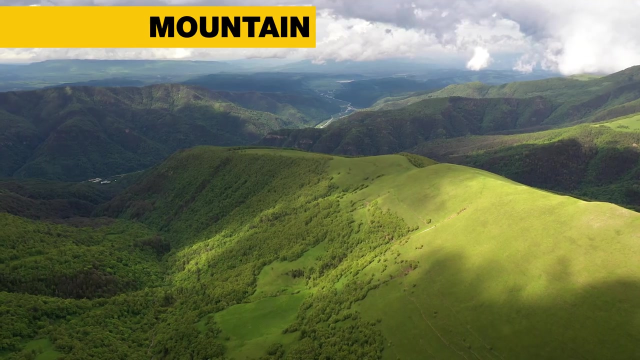 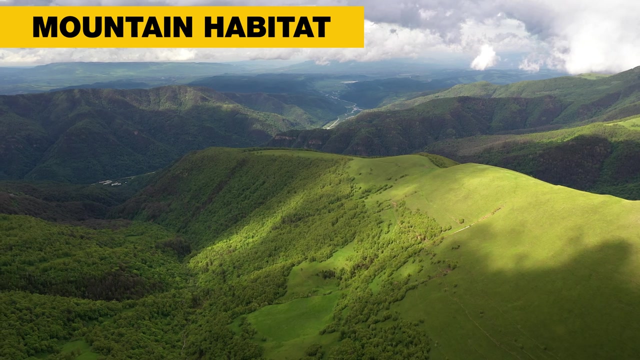 Penguin, Polar Bear, Arctic Fox, Leopard Seal, Snowy Owl, Albatross, Reindeer, Reindeer Mountain, Habitat Mountain. Habitat Mountains are home to plants and animals that are adapted to the very harsh weather conditions they experience. Most of the time it is cold and windy. 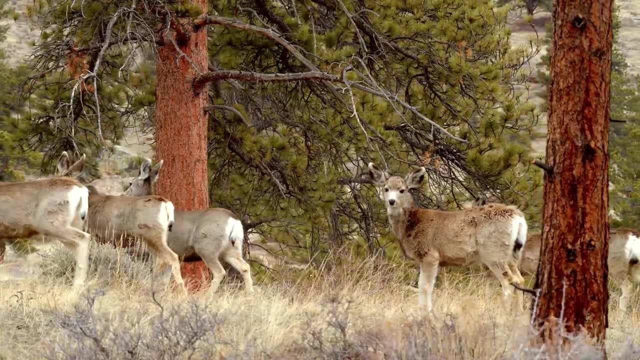 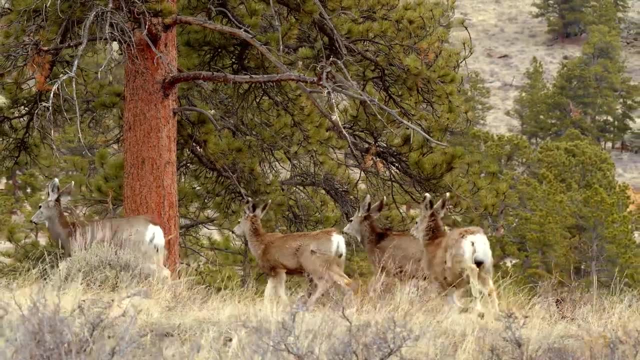 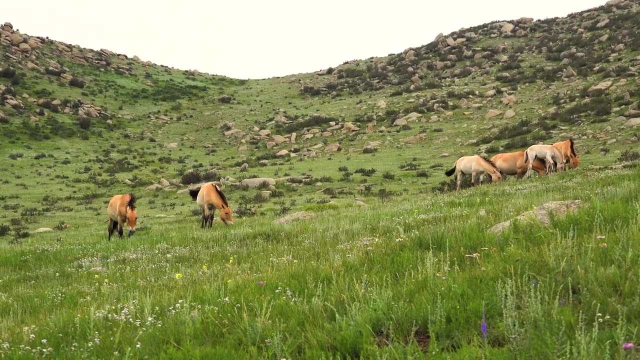 The lower slopes of a mountain ecosystem are usually covered with forests, But as you go higher in the mountains, the air gets thinner, colder and less oxygen is available. Some plants do not survive at high altitudes because they require warm temperatures to grow. 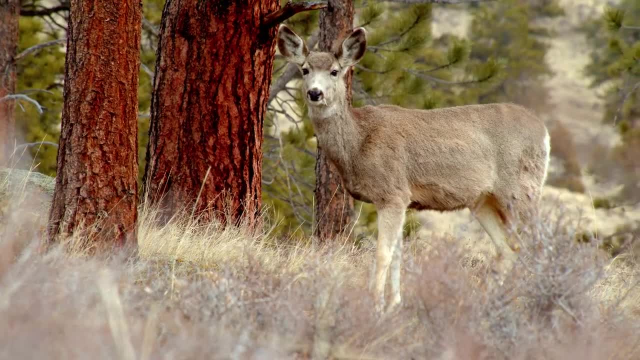 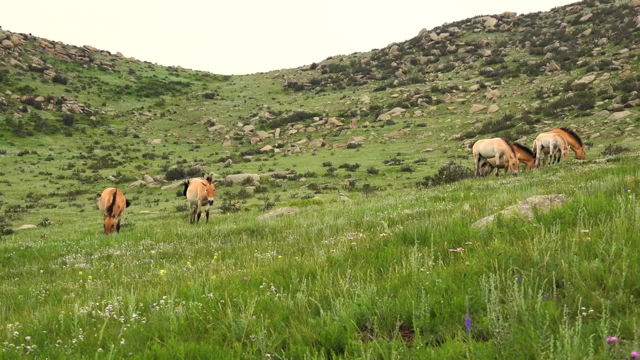 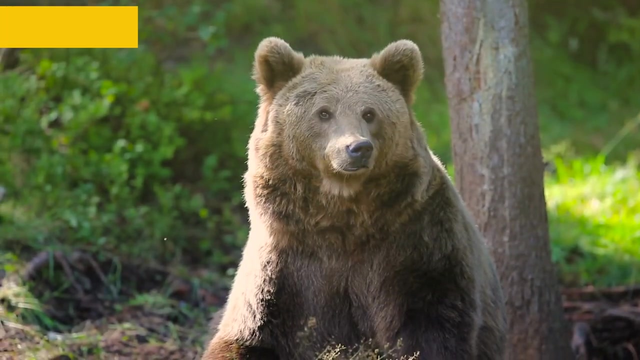 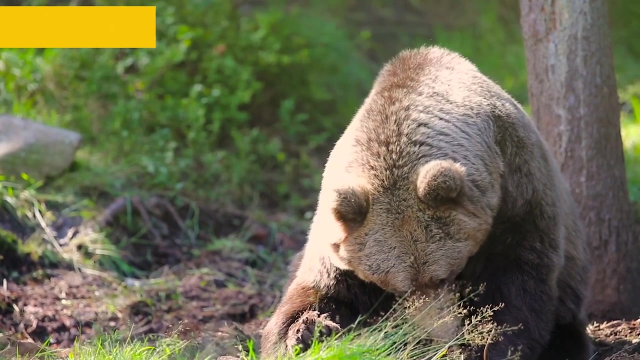 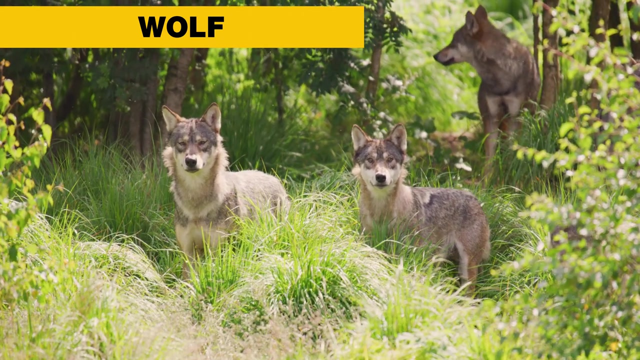 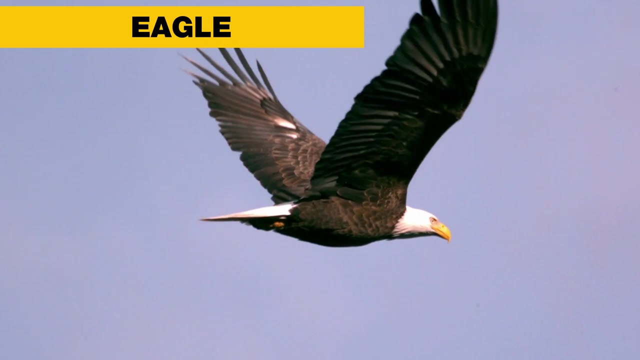 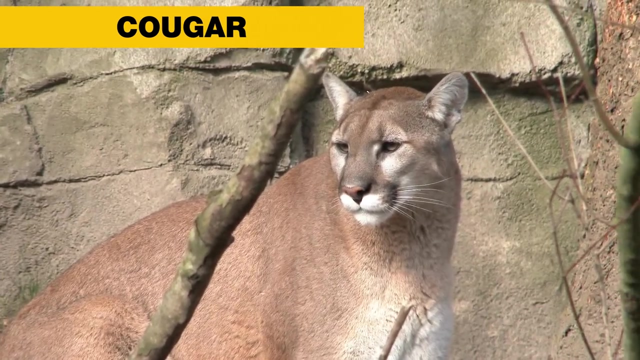 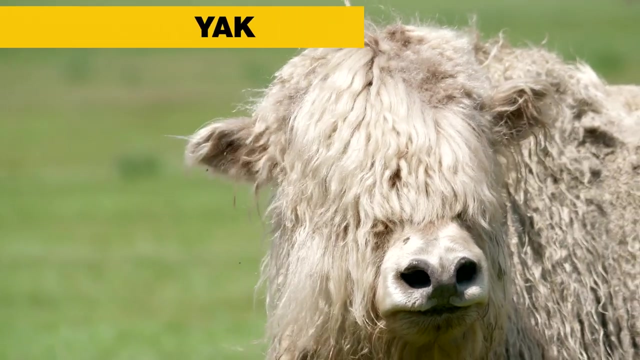 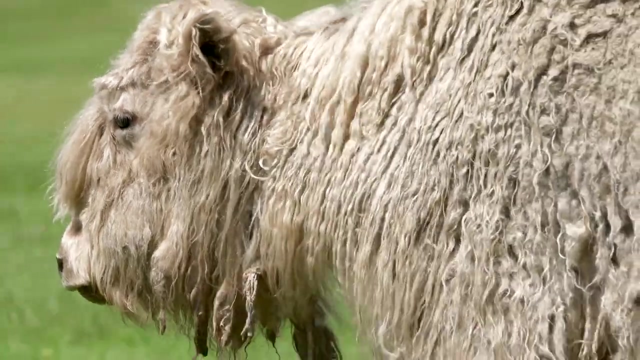 Most freshwater streams, lakes and rivers originate from melting snow, or glaciers come from mountain habitats. Here are some animals that live in mountains: Brown Bear, Wolf, Eagle, Cougar, Cougar, Monk, inconspicuous Jack, Goat, Crane, Yellow desert horse, Big Horned Yourbo. 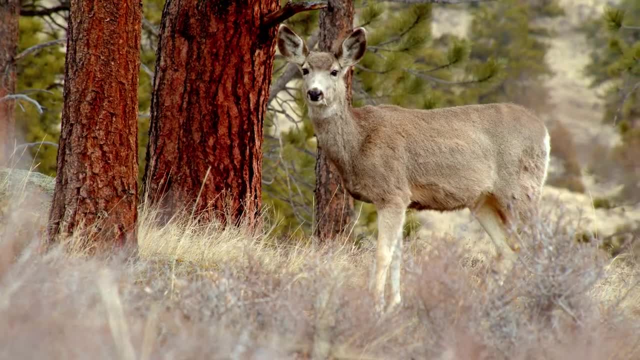 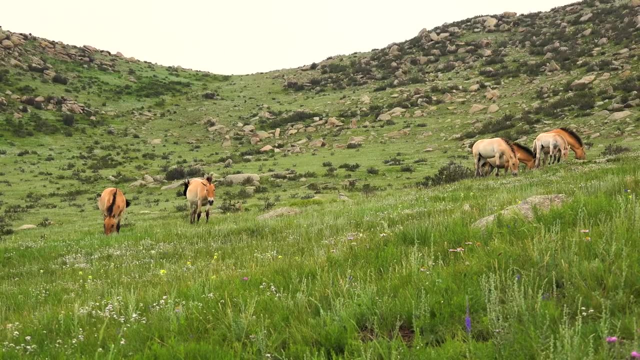 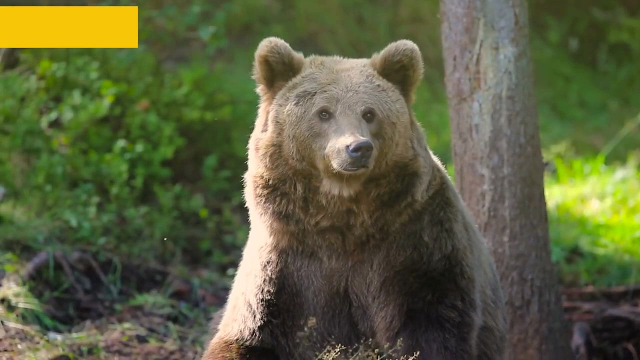 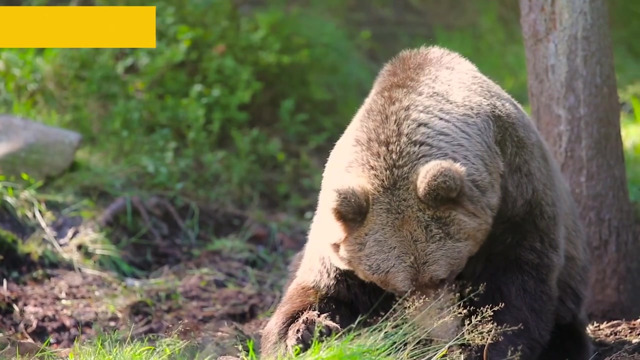 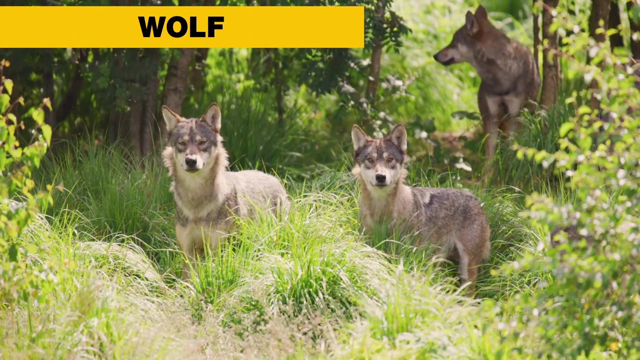 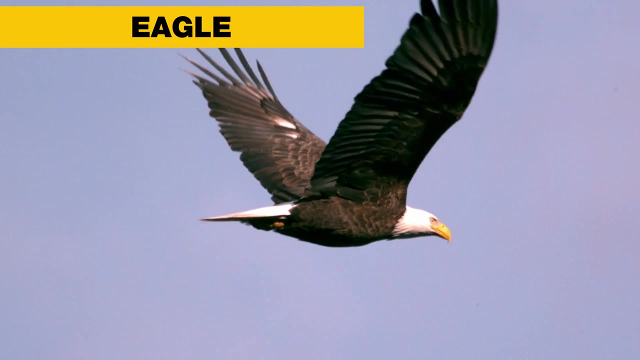 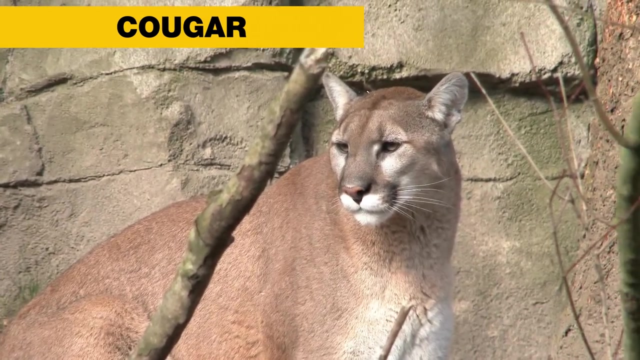 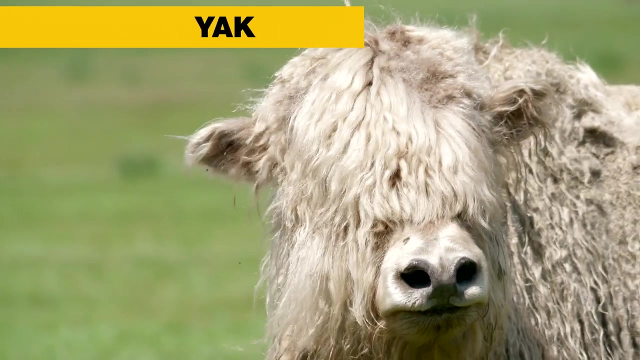 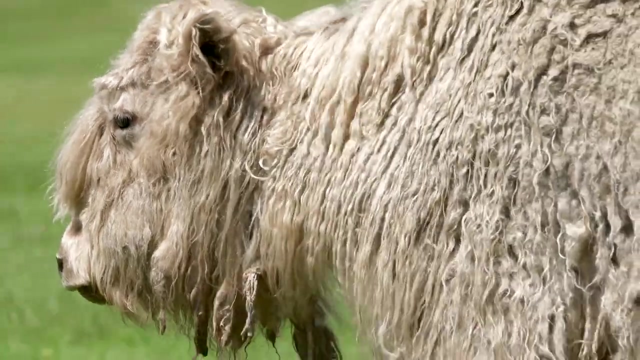 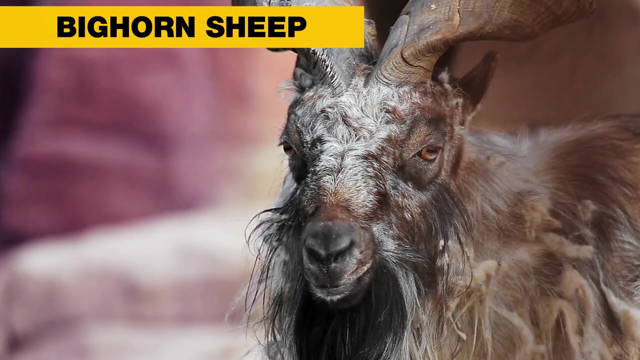 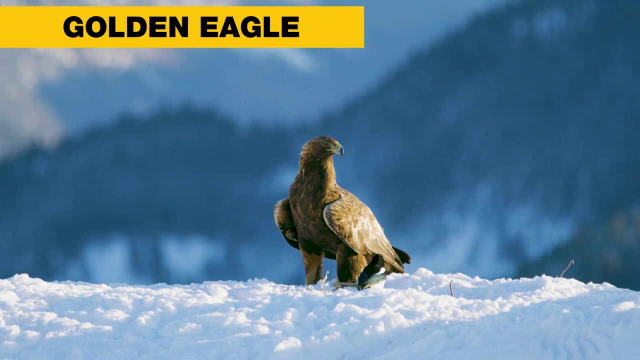 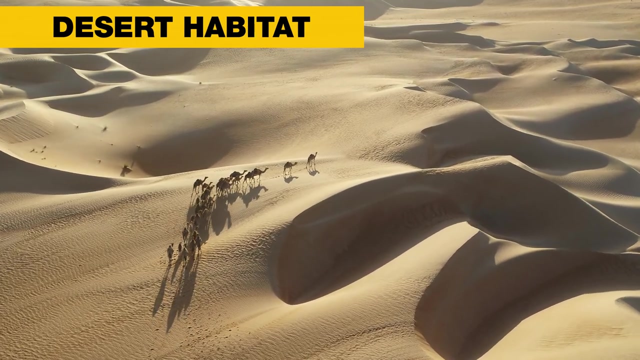 Most freshwater streams, lakes and rivers originate from melting snow, or glaciers come from mountain habitats. Here are some animals that live in mountains: Brown Bear, Wolf Eagle, Cougar, Cougar Bush, Ox Eagle, Apple, сhiro Eagle, Golden Eagle, Chicken. Deserts are areas that have extreme and long periods of dry weather. 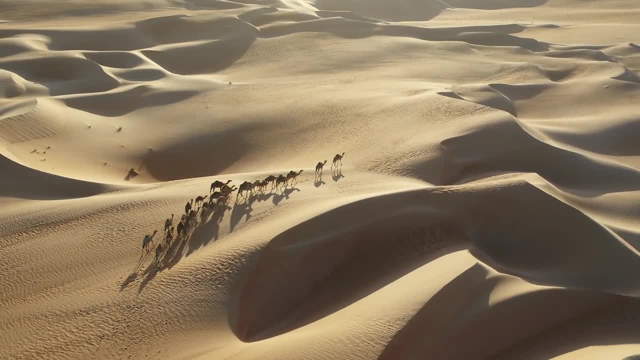 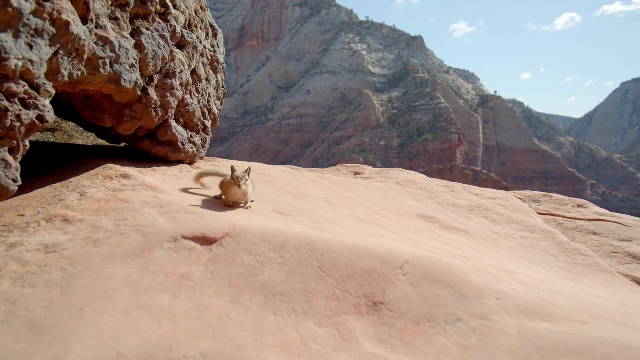 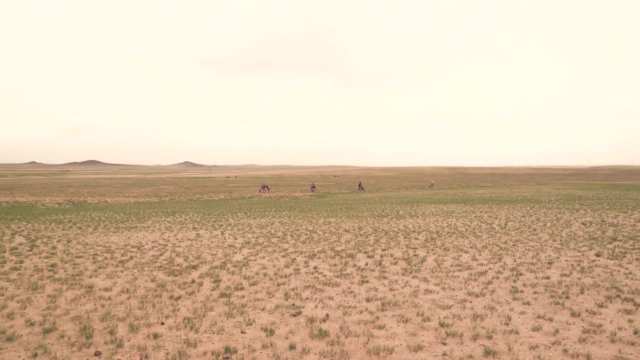 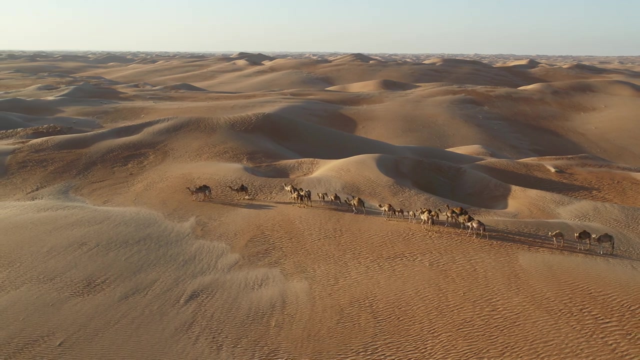 Deserts are characterized by extreme heat and cold, wind, sandstorms and minimal animal life. The temperature difference between day and night is enormous, Although it is not very hot and rainy. some animals survive in this habitat, As a desert is deprived of water. many adaptations, like thick leaves, deep roots and flexible 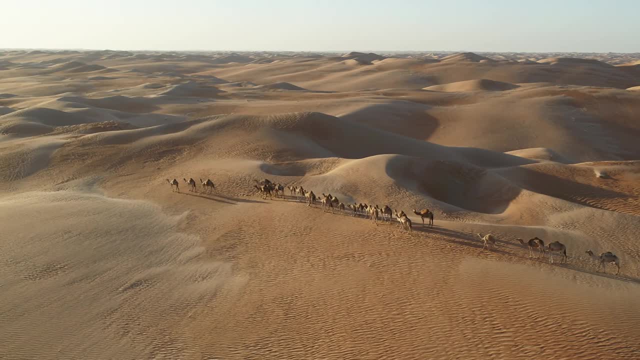 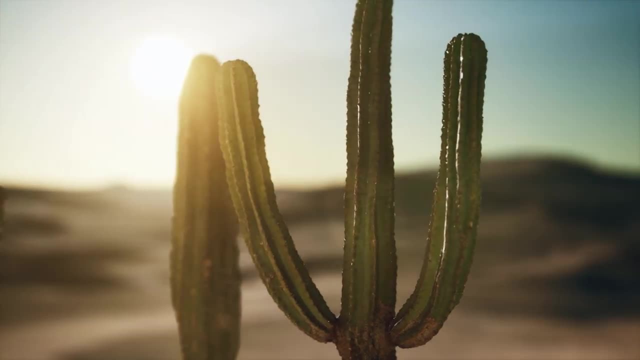 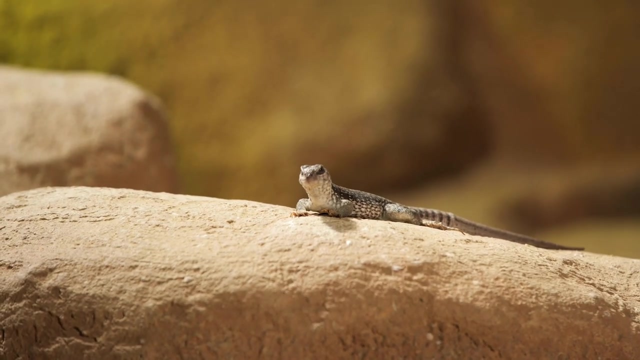 stems allow desert plants to survive. Some plants also have adaptations to store water, such as cactuses. There are several animals living in the desert too, comprising some unique species, Animals such as camels, lizards and antelopes. 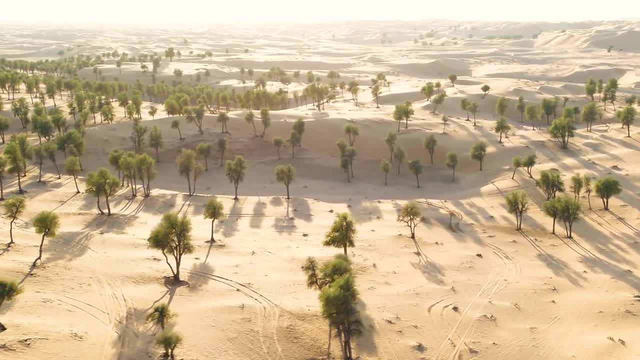 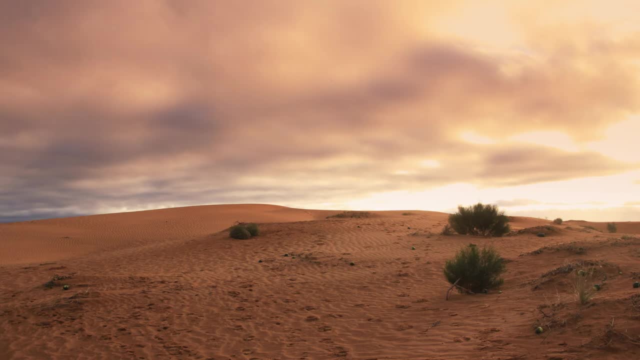 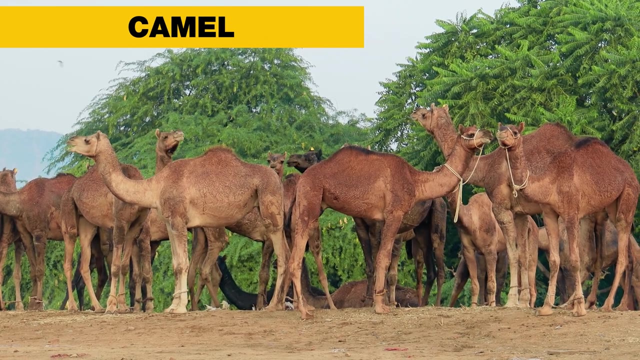 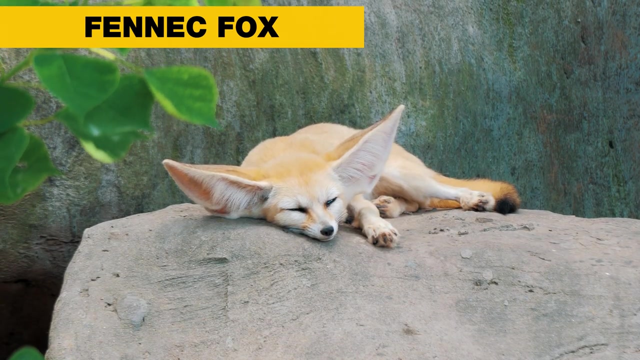 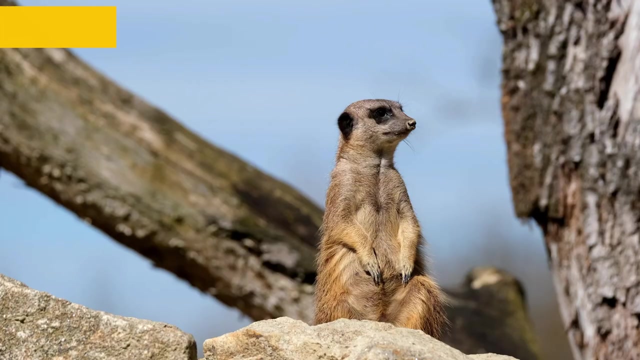 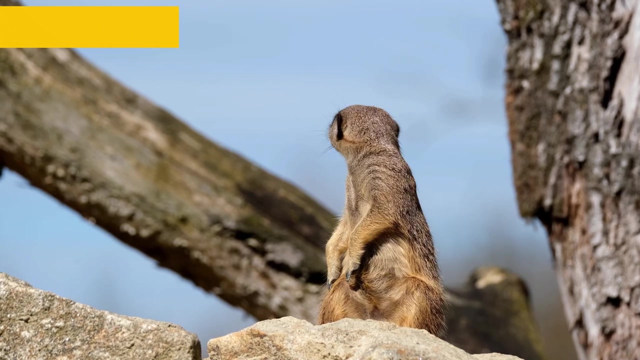 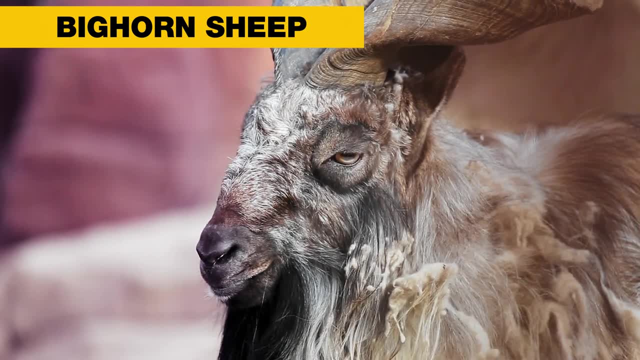 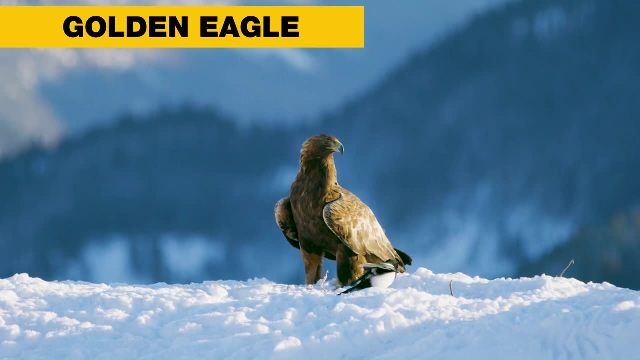 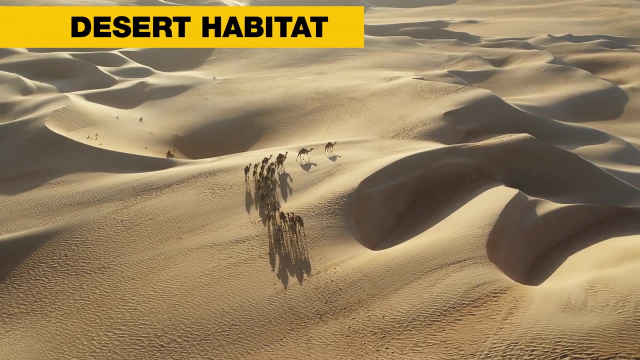 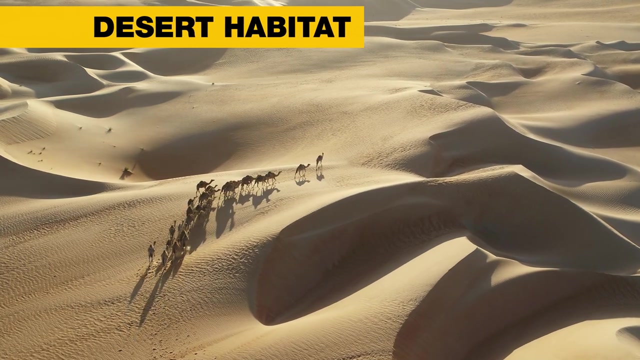 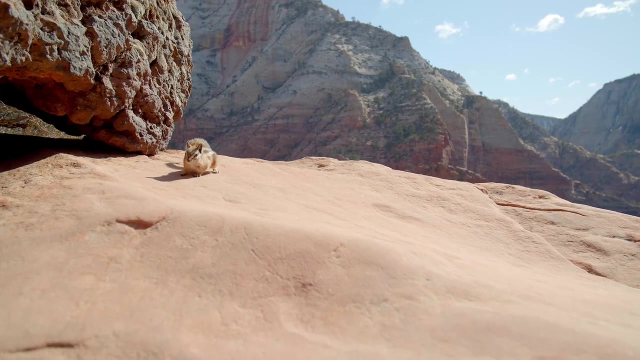 F deh- Toothless Wild Chasing Deserts are areas that have extreme and long periods of dry weather. Deserts are characterized by extreme heat and cold wind, sandstorms and minimal animal life. The temperature difference between day and night is enormous. 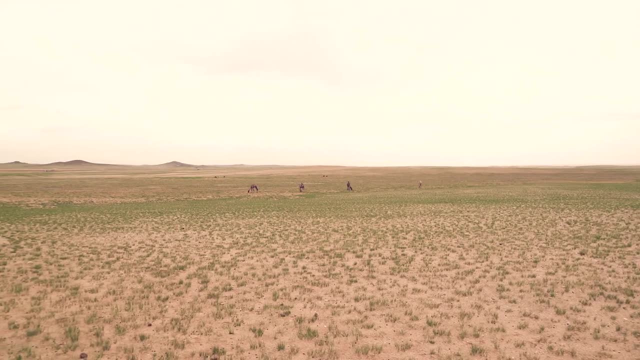 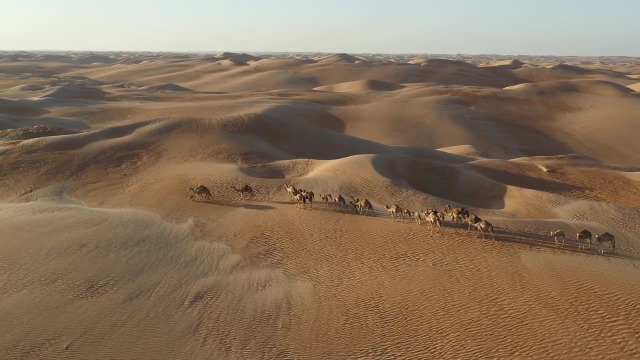 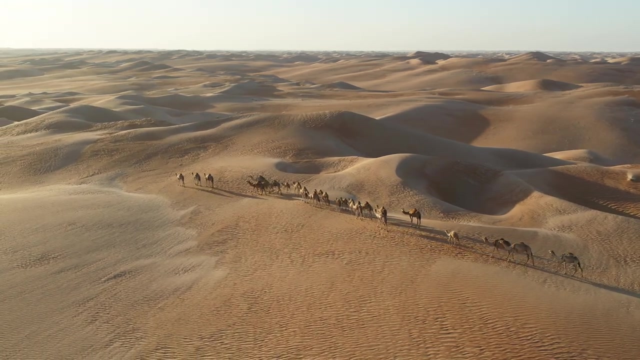 Although it is not very hot and rainy, some animals survive in this habitat, As a desert is deprived of water. many adaptations, like thick leaves, deep roots and flexible stems, allow desert plants to survive. Some plants also have adaptations to store water, such as cactuses. 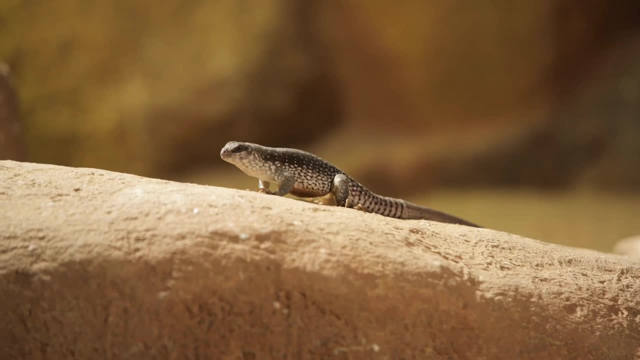 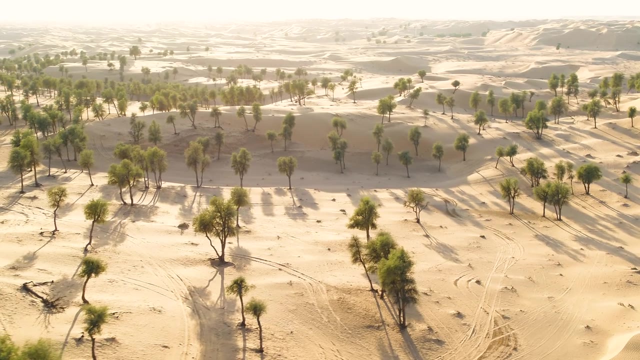 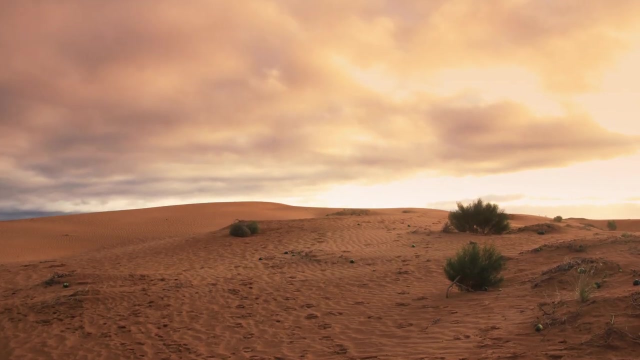 There are several animals living in the desert too, comprising some unique species, Animals such as camels, lizards and antelopes. Camels have special adaptations that enable them to thrive under tough conditions such as minimal food availability or extreme temperatures. 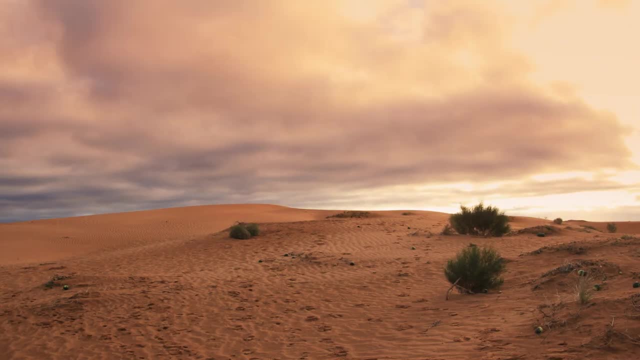 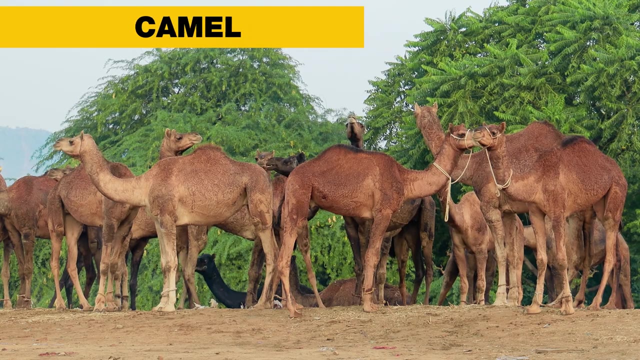 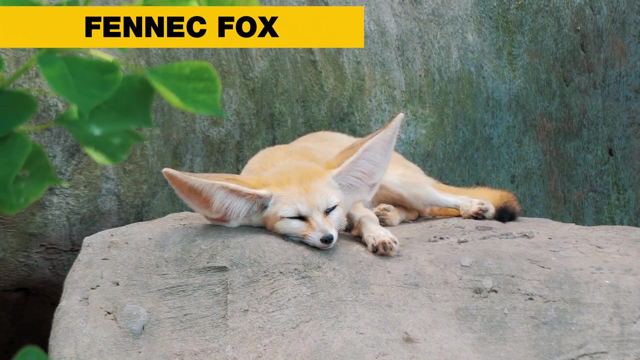 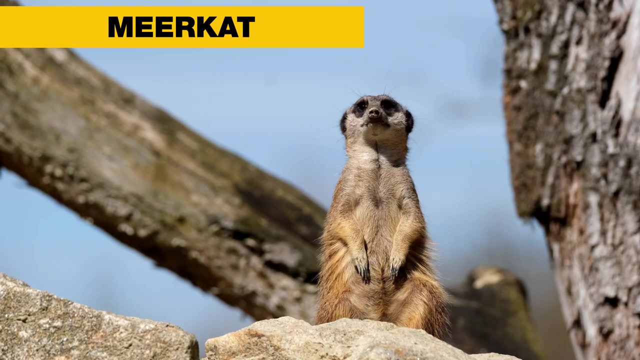 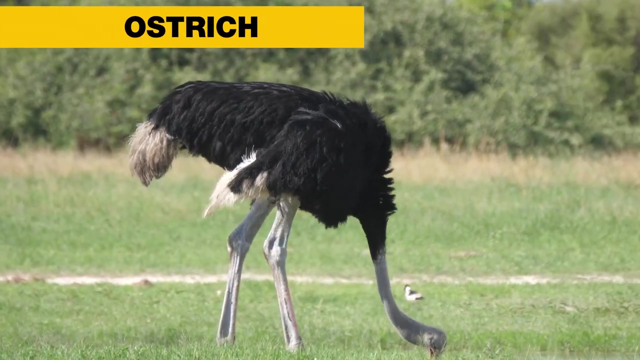 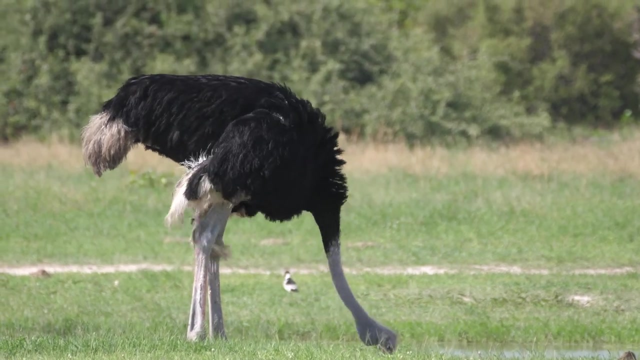 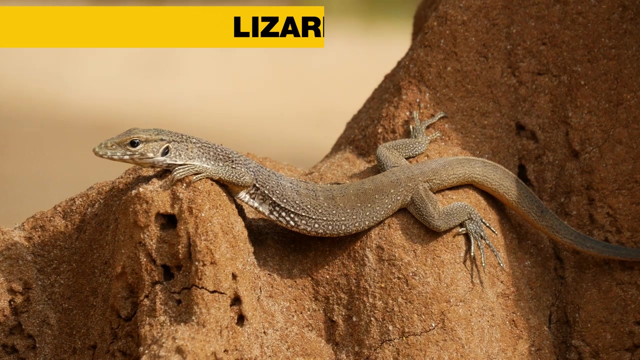 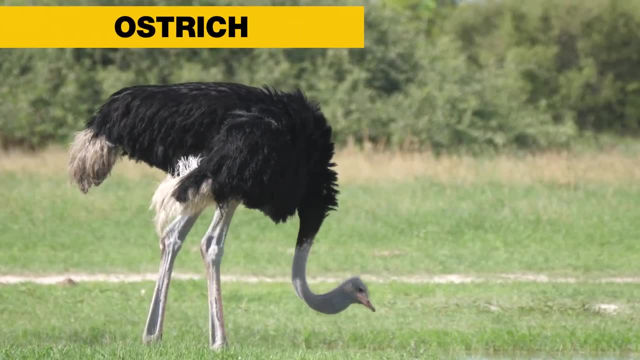 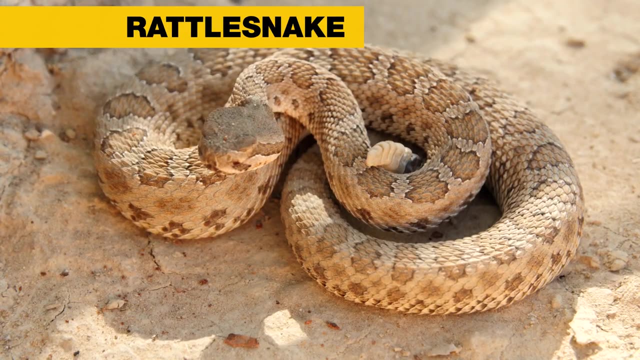 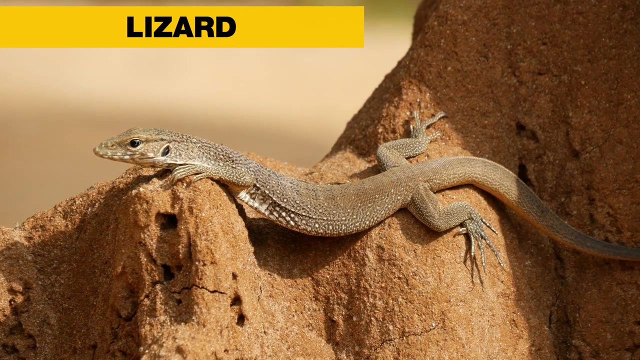 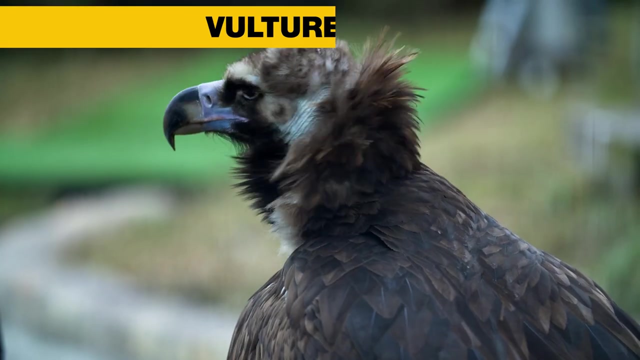 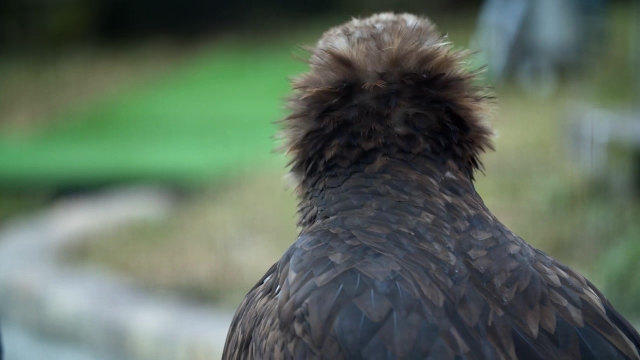 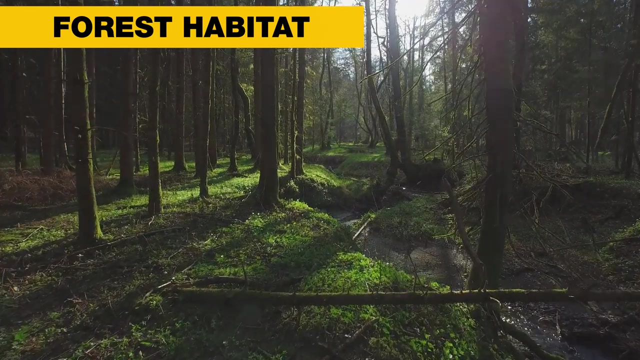 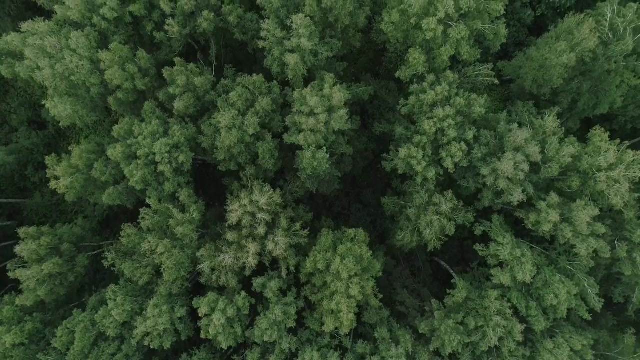 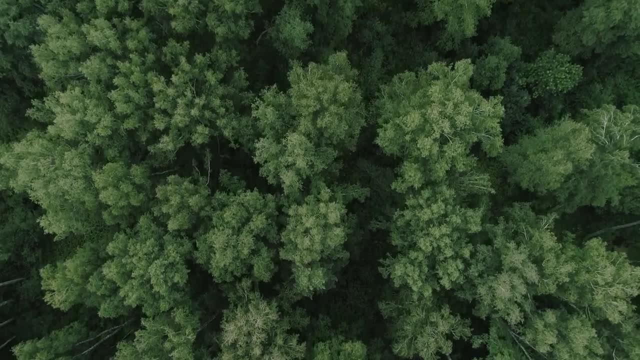 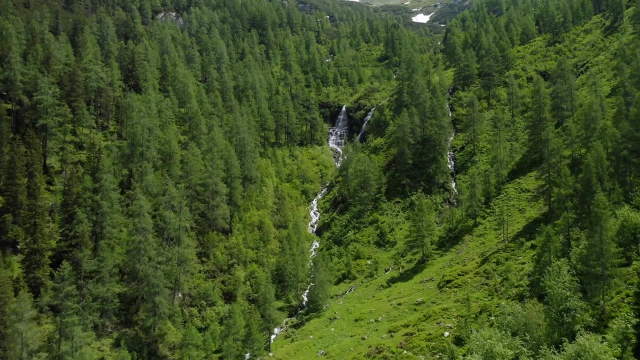 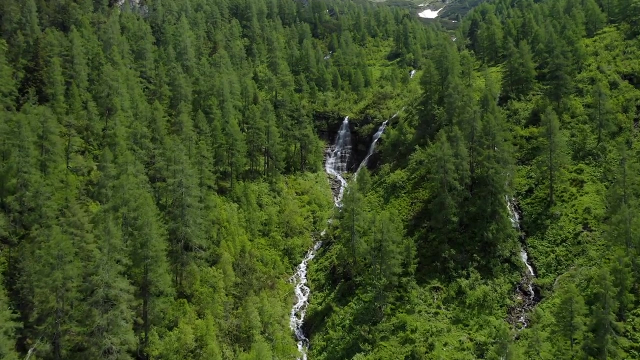 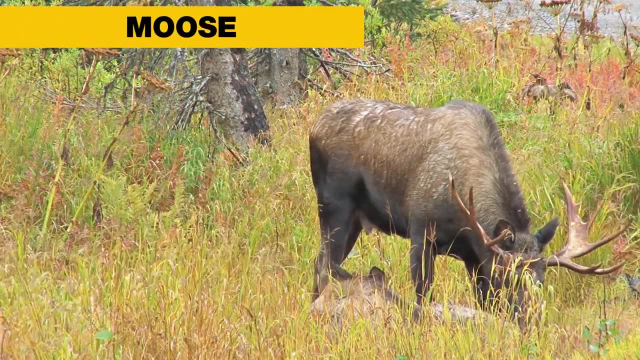 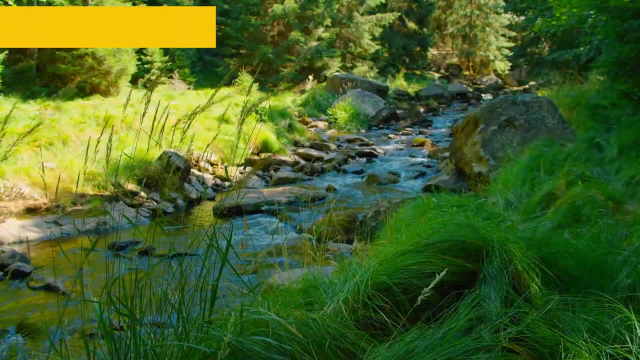 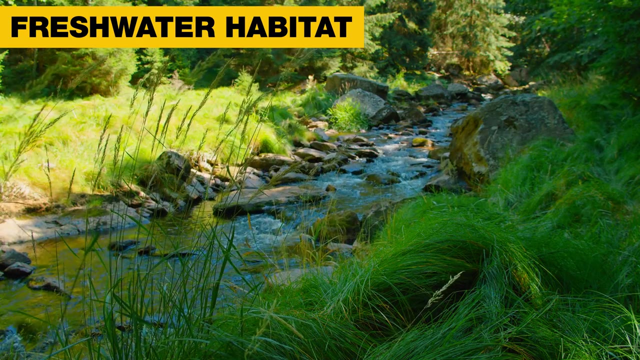 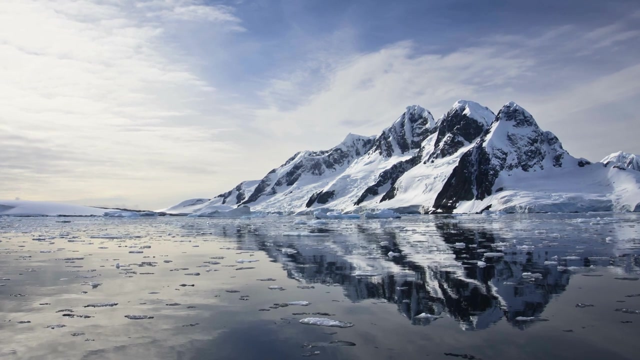 Woodpecker, émous, Woodpecker, Woodpecker, elling Moose Freshwater Habitat. Freshwater habitat covers about 20% of the world and is found in various parts. proportion of freshwater in the world, Because as you go from the equator to the poles, 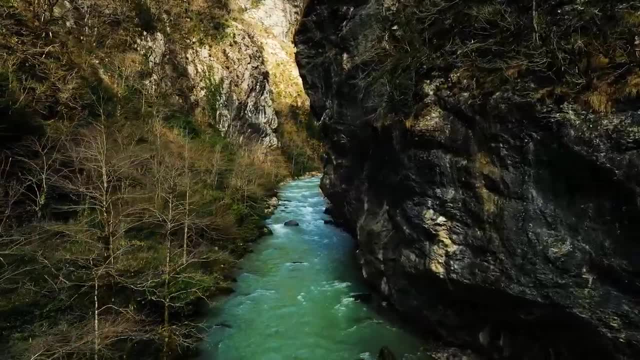 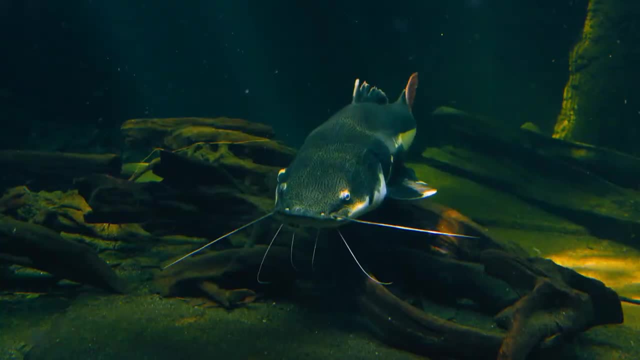 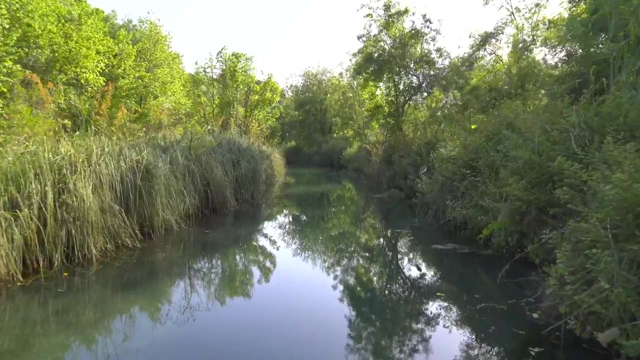 the salinity of the seas decreases. That's why glaciers are considered freshwater. Glaciers are followed by lakes, rivers, streams, groundwater and dams. Freshwater habitats are not evenly distributed across the globe. For example, while freshwater resources are sufficient in the Americas, 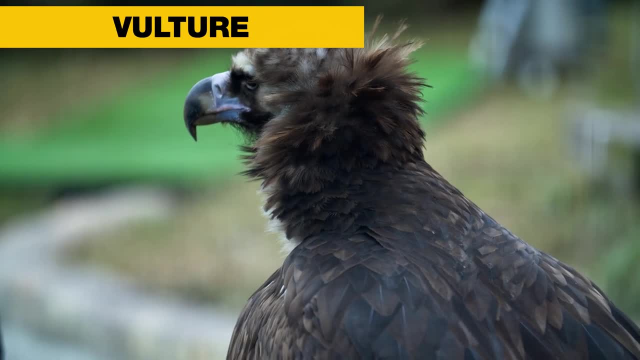 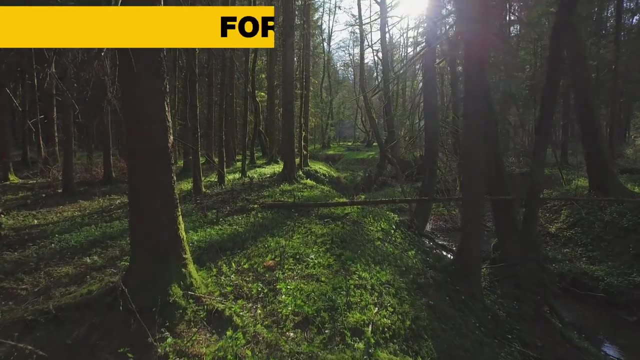 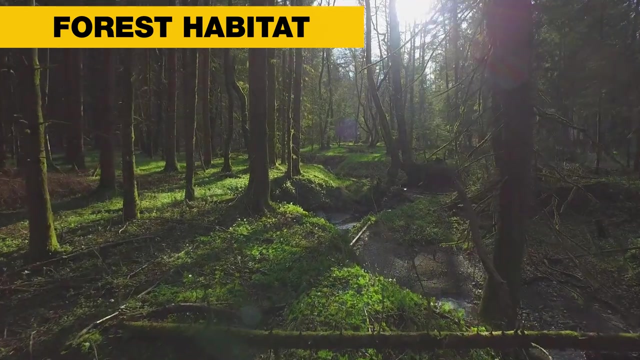 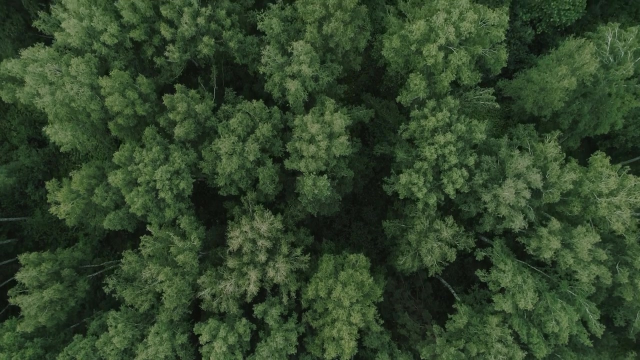 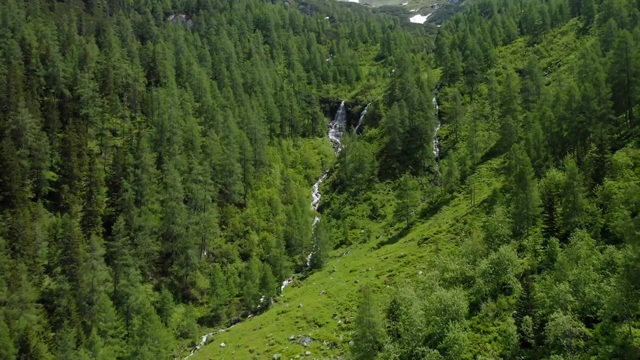 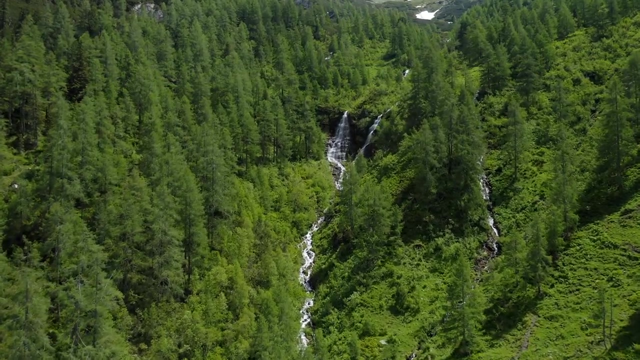 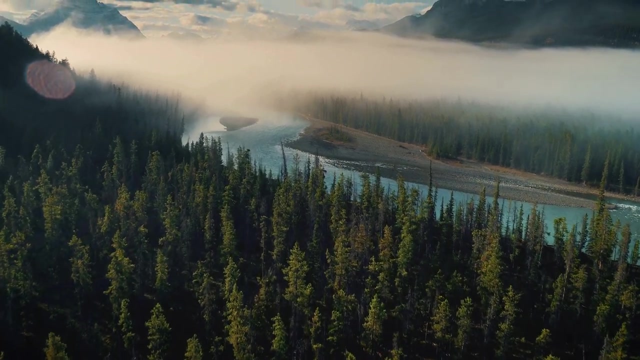 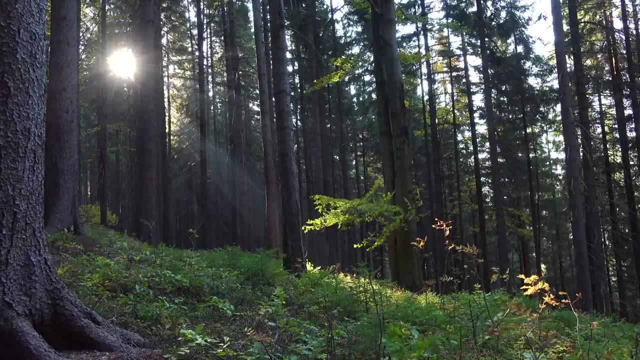 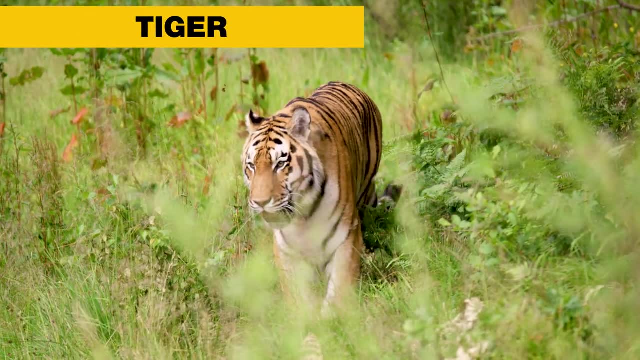 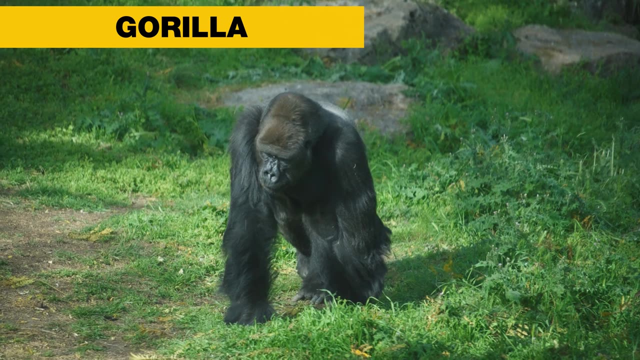 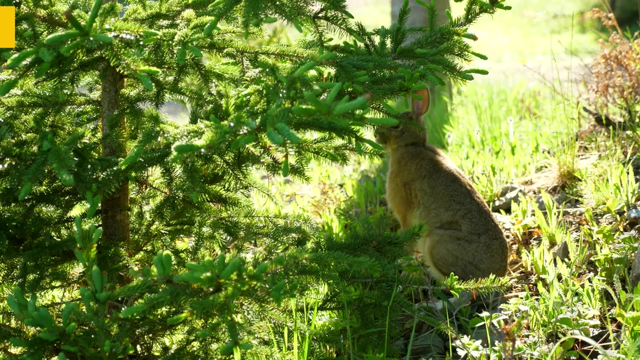 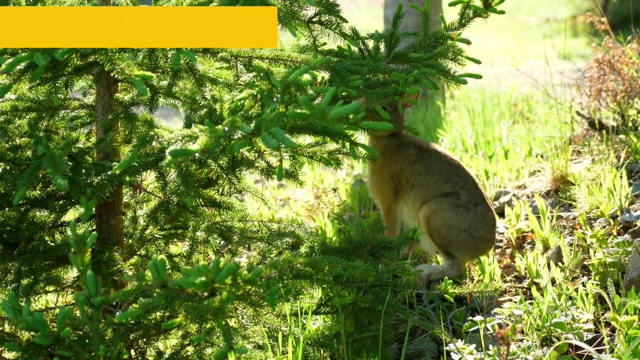 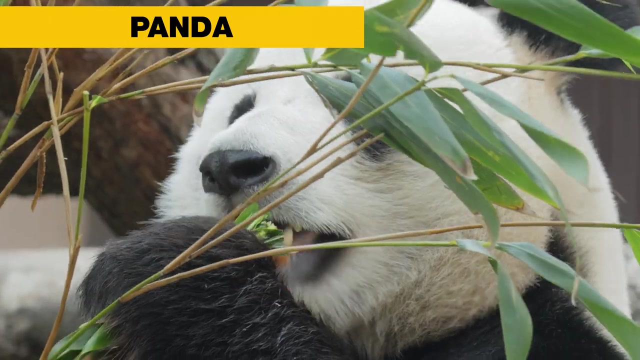 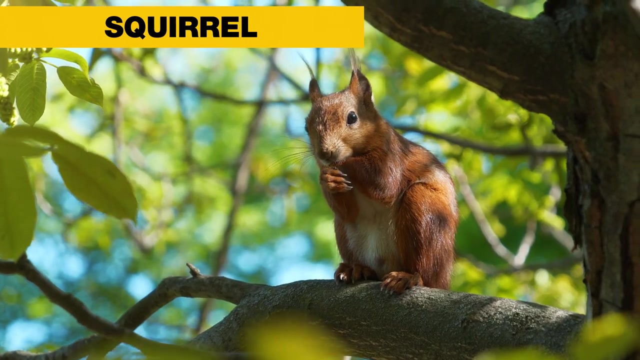 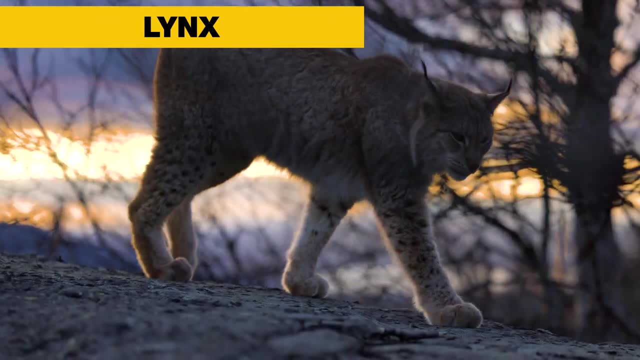 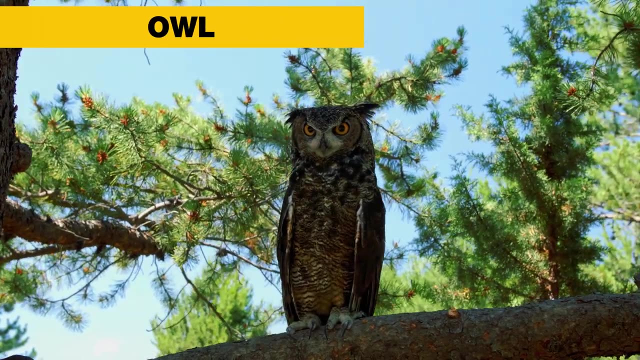 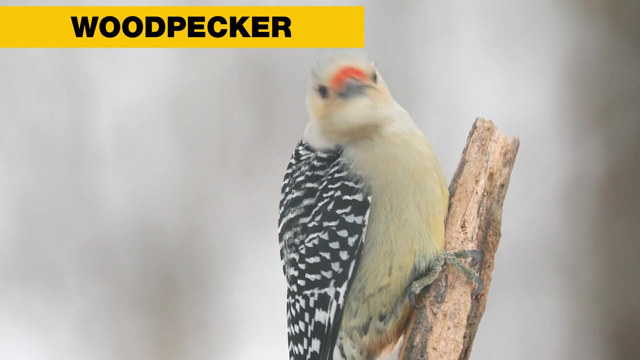 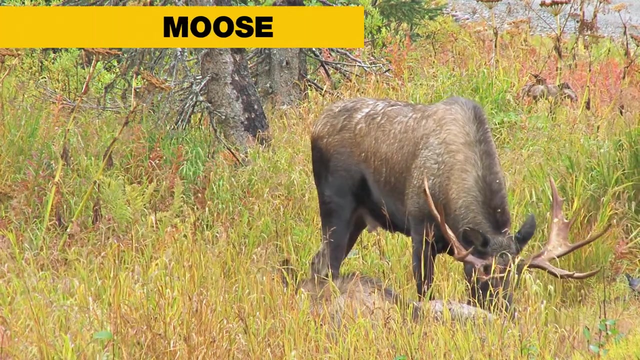 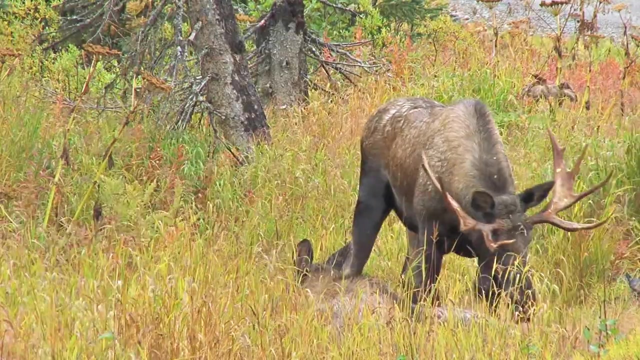 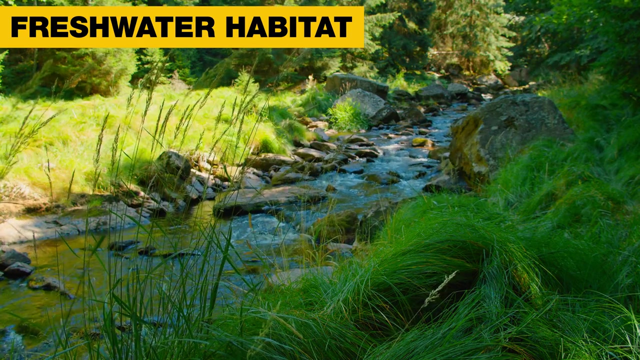 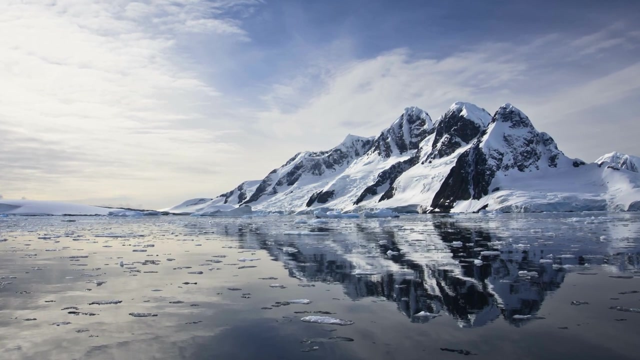 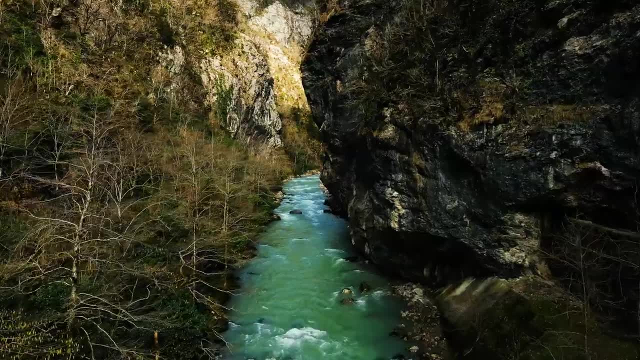 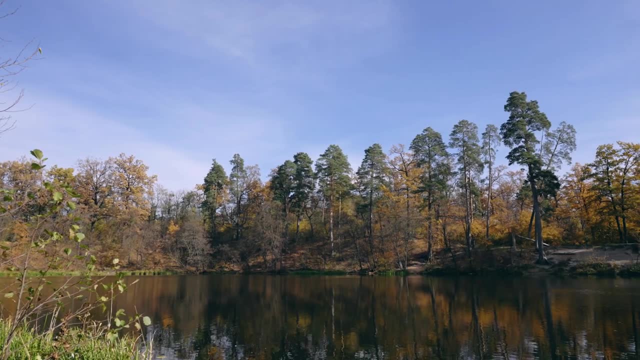 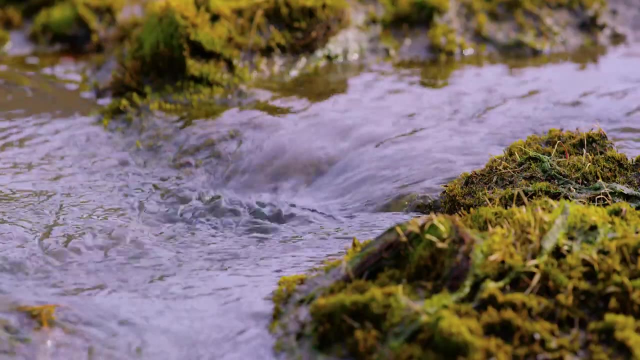 Because, as you go from the equator to the poles, the salinity of the seas decreases. That's why glaciers are considered freshwater. Glaciers are followed by lakes, rivers, streams, groundwater and dams. Freshwater habitats are not evenly distributed across the globe. 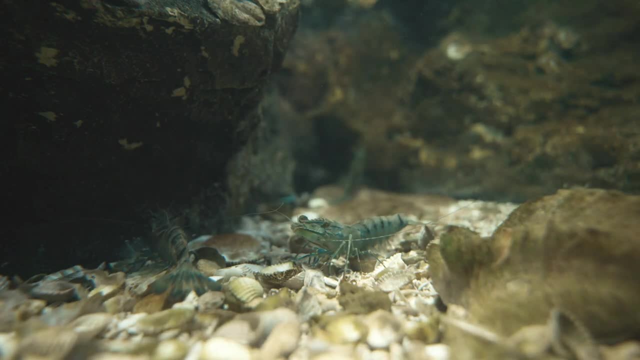 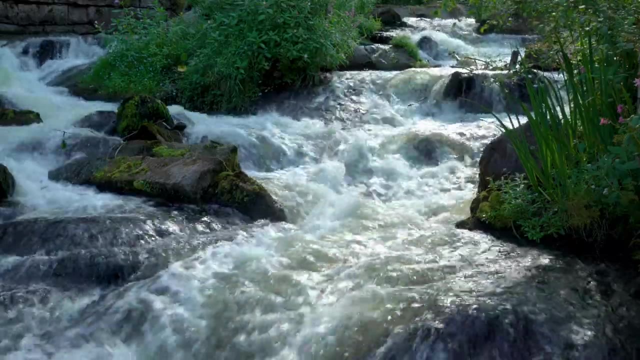 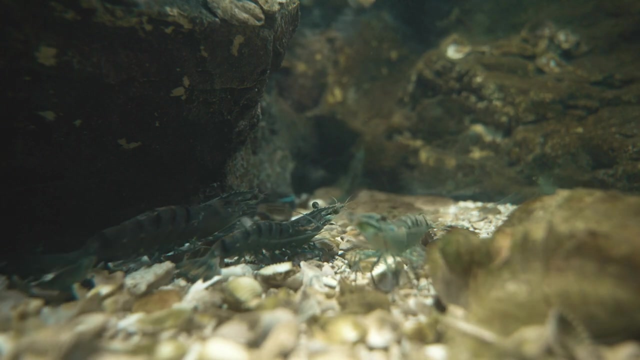 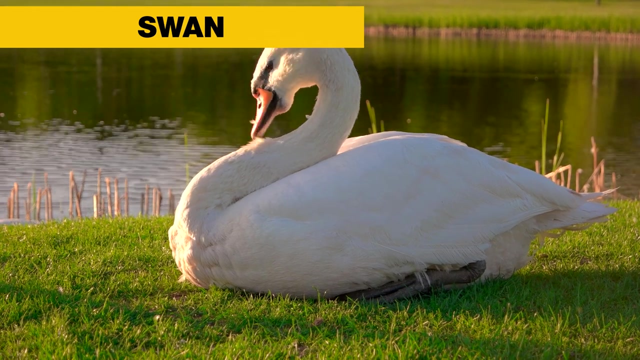 For example, while freshwater resources are sufficient in the Americas, they are quite limited in Northern Africa. Freshwater habitats are home to numerous animal and plant species and provide us with water and food. Here are some animals that live in freshwater habitats: Swan Beaver. 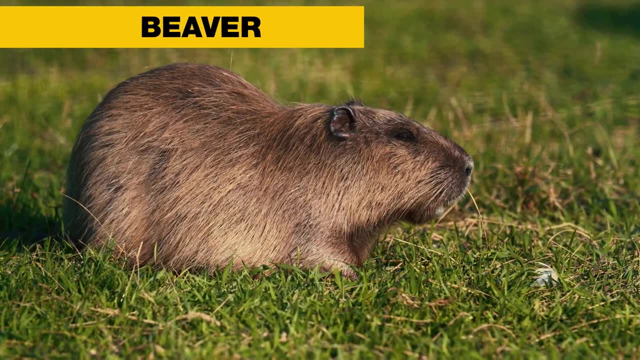 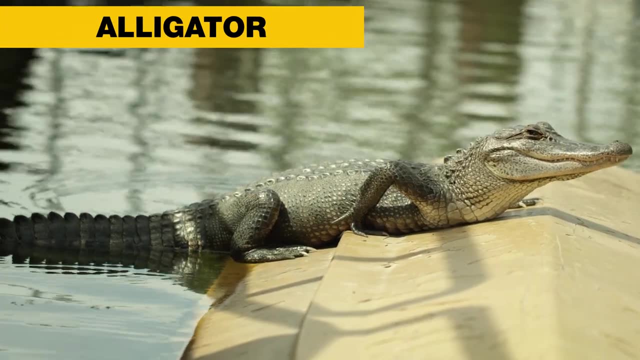 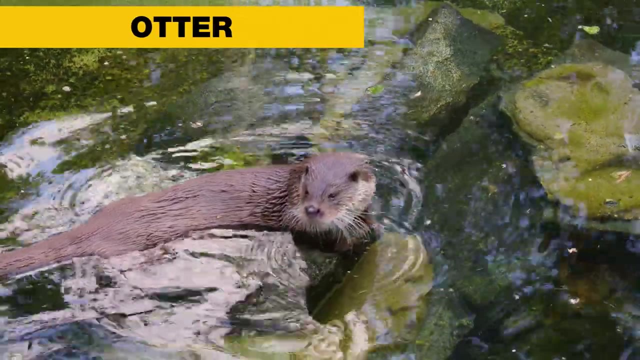 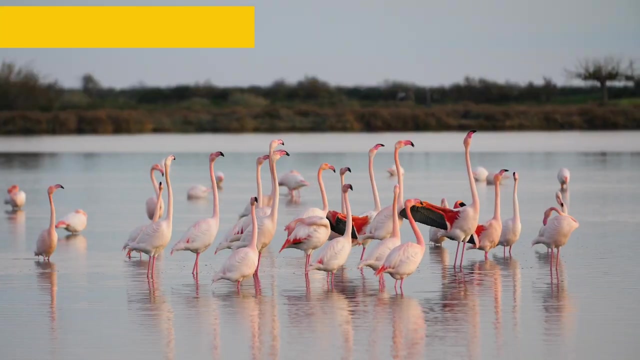 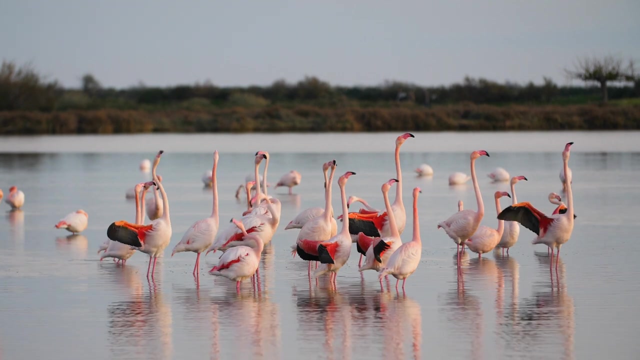 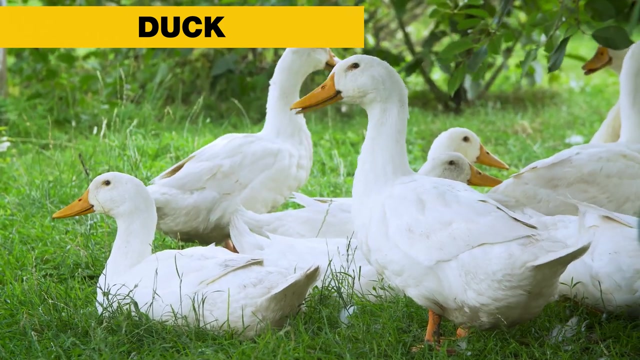 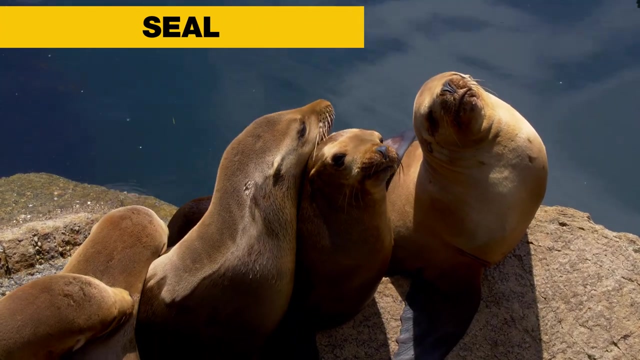 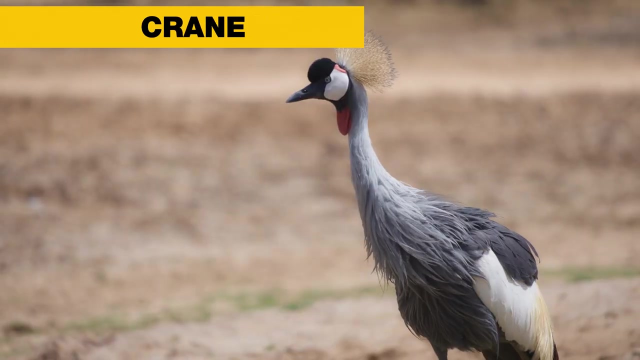 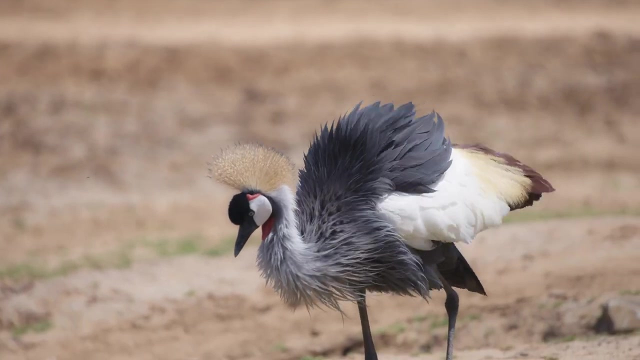 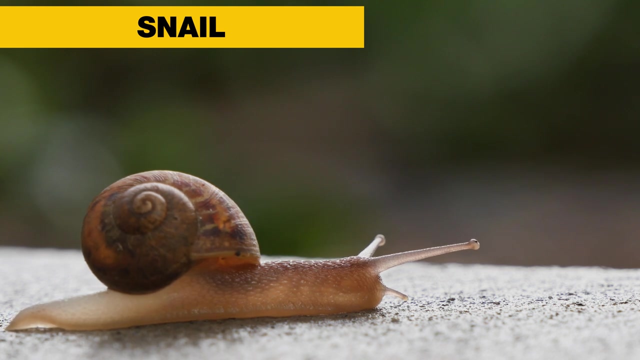 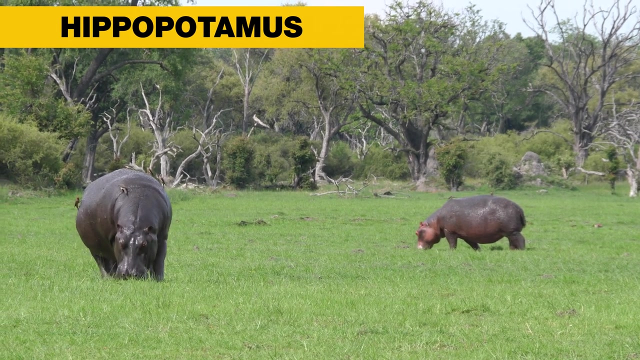 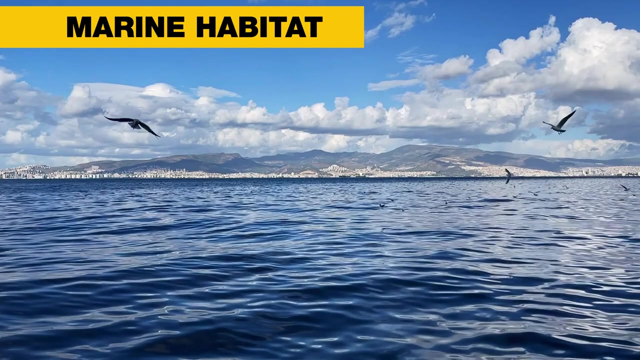 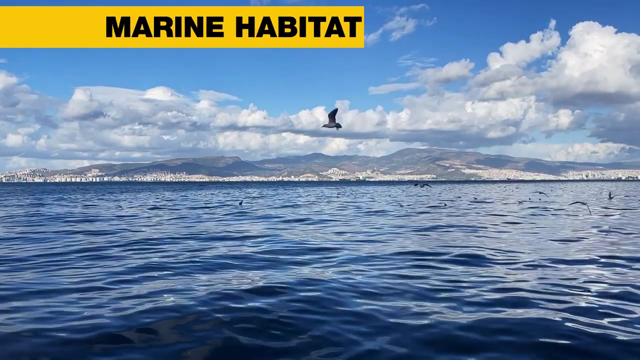 Alligator Otter, Flamingo Caterpillar, Caterpillar Caterpillar Caterpillar Duck Roach, Duck Seal Crane, Cran Crane Crane Crane Crane, Crane Crane, Snail Hippopotamus Marine Habitat. The marine habitat consists primarily of saltwater oceans. It is the largest habitat on planet Earth and covers about 70% of the Earth's surface. 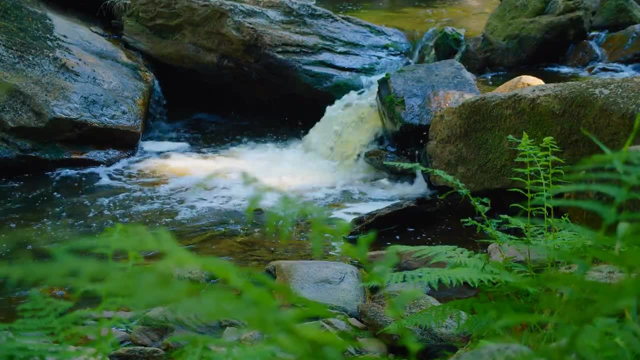 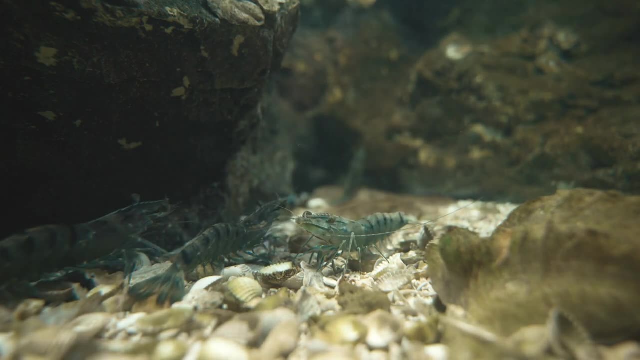 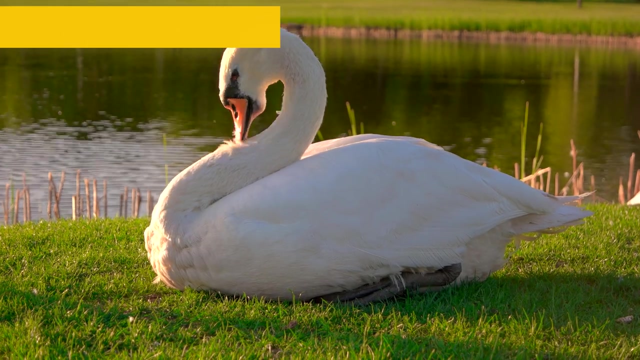 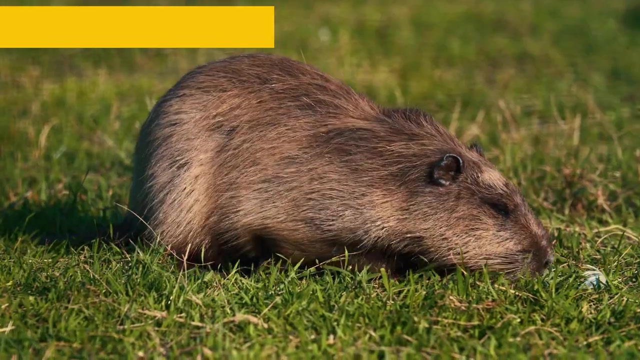 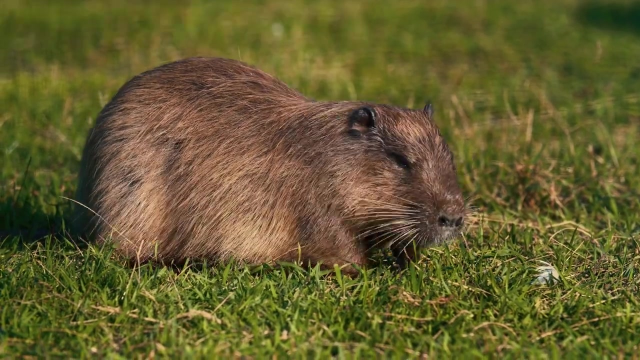 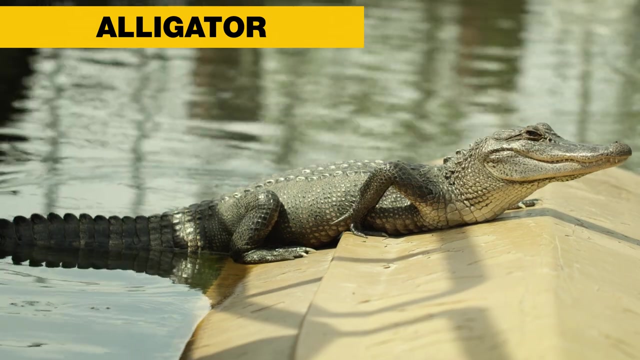 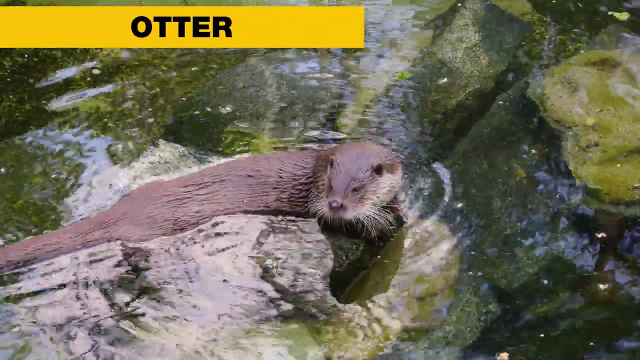 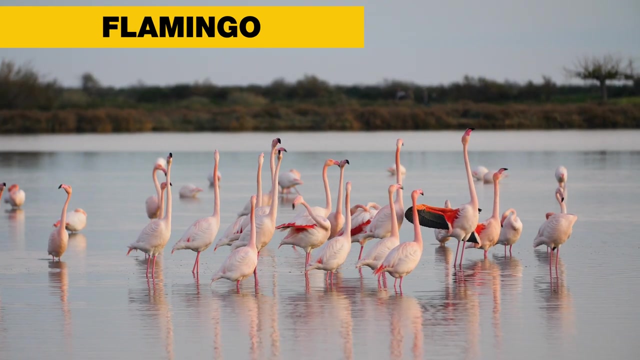 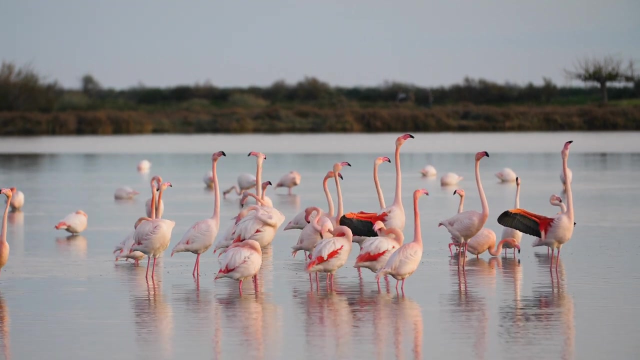 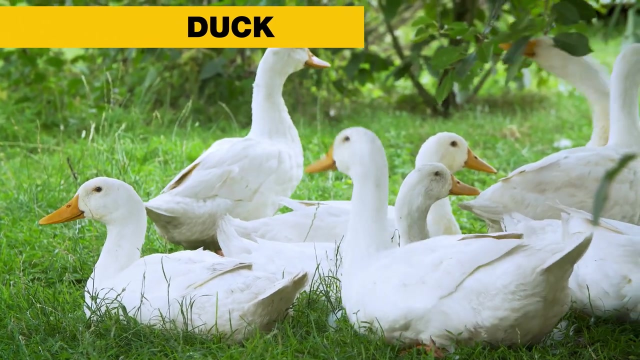 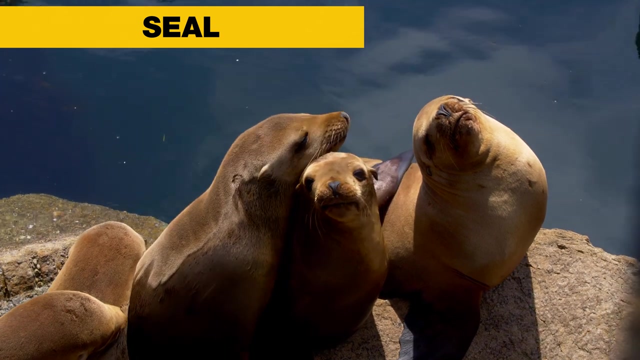 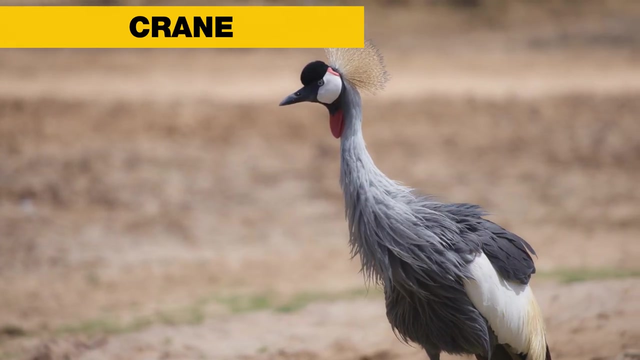 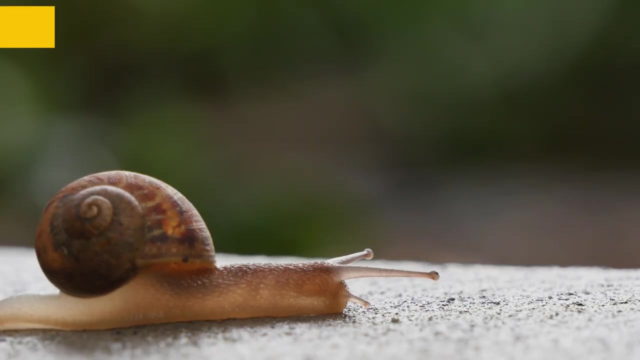 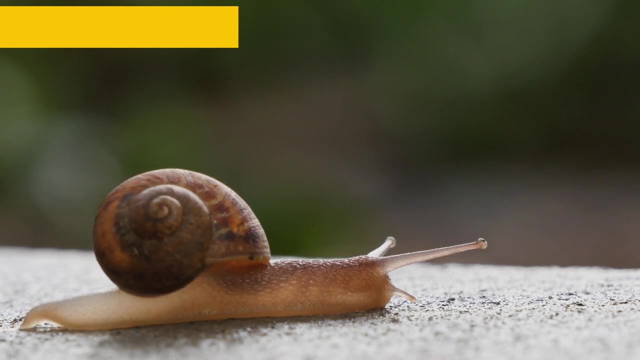 they are quite limited in Northern Africa. Freshwater habitats are home to numerous animal and plant species and provide us with water and food. Here are some animals that live in freshwater habitats: Swan, Beaver, Alligator, Otter, Flamingo, Duck, Seal, Crane, Snail. 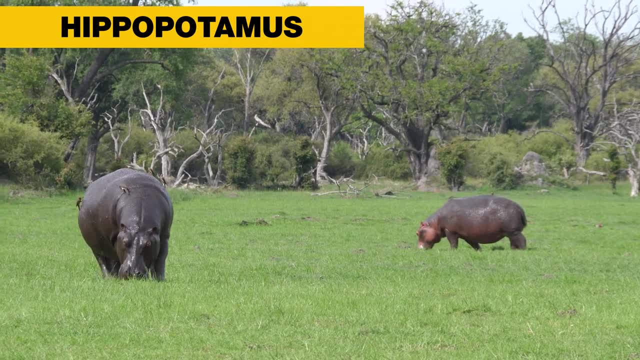 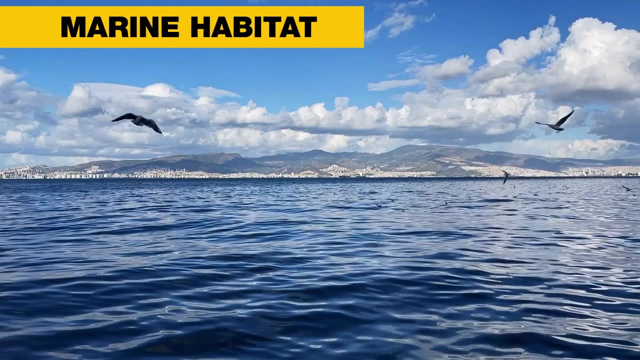 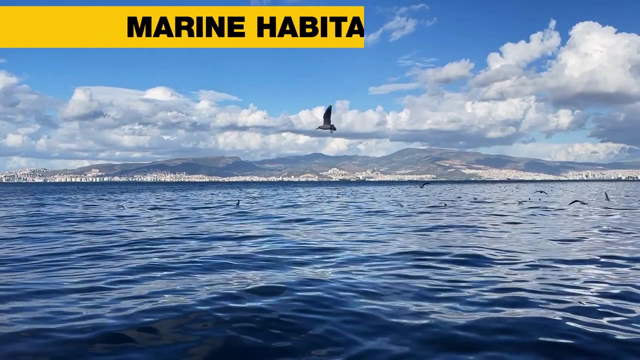 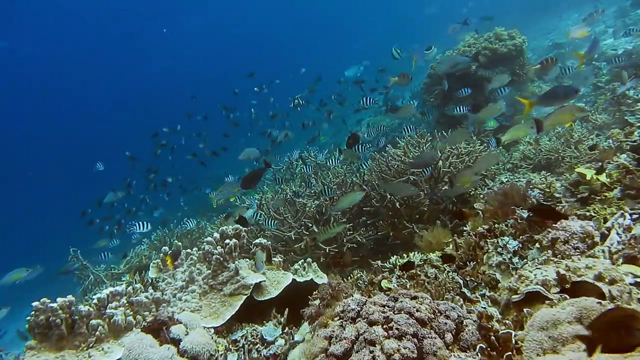 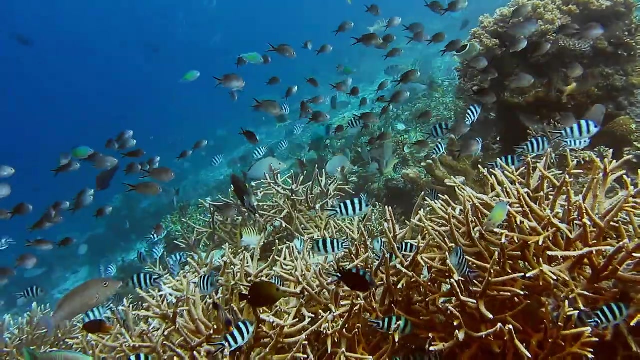 Hippopotamus Marine Habitat. The marine habitat consists primarily of saltwater oceans. It is the largest habitat on planet Earth and covers about 70% of the Earth's surface. The marine habitat is the most biodiversity of all habitats. Here are some animals that live in marine habitats. 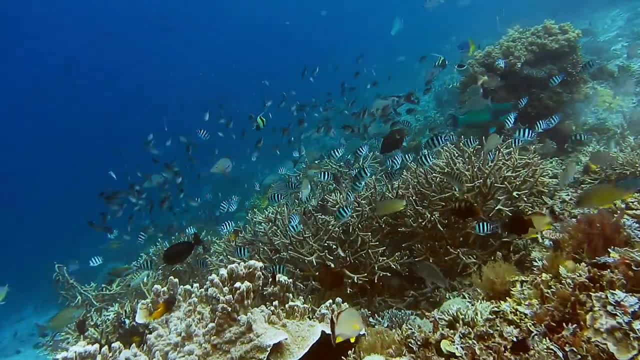 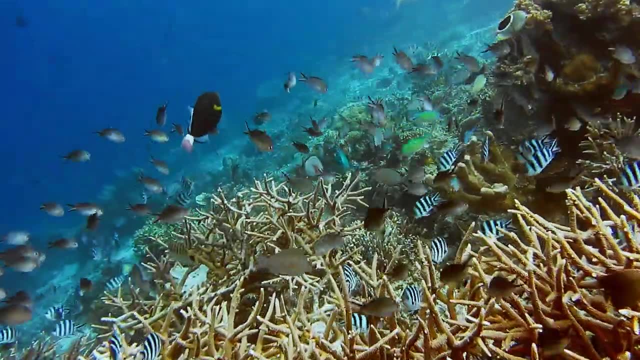 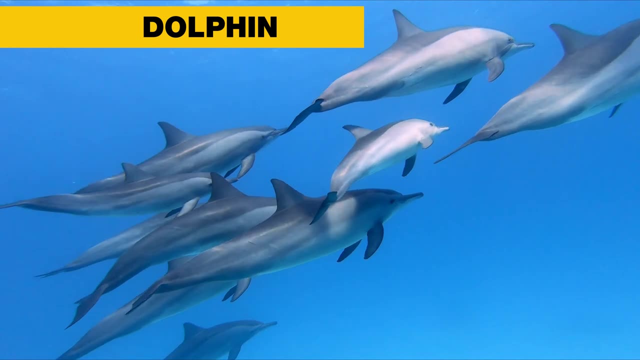 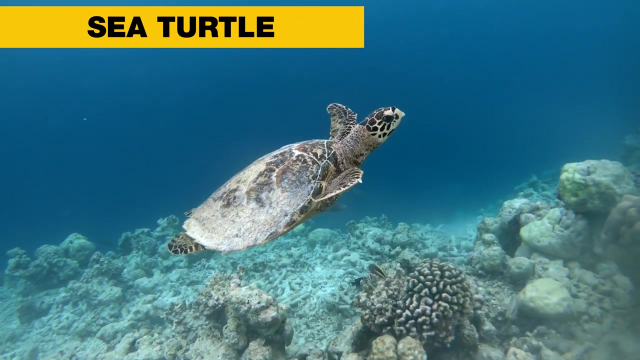 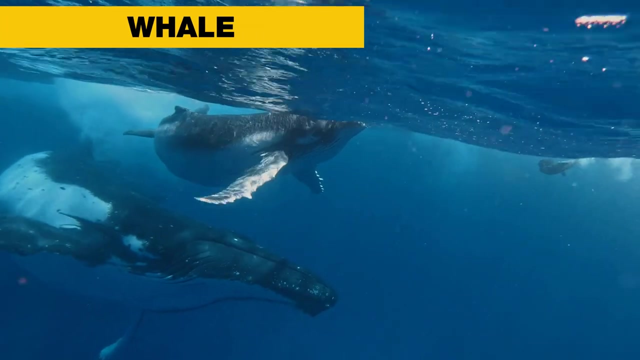 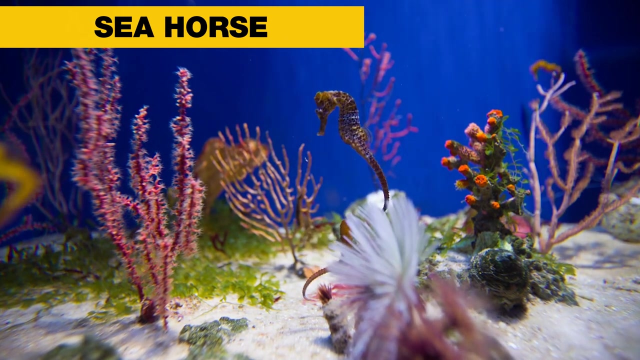 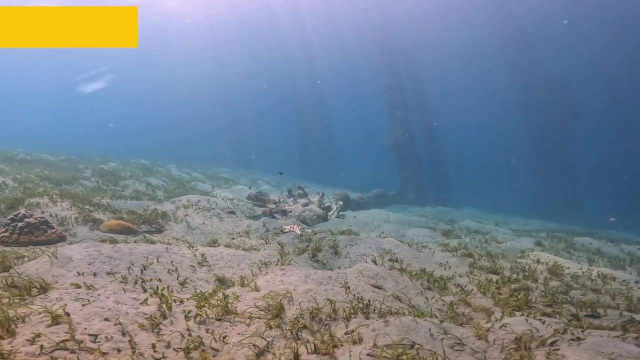 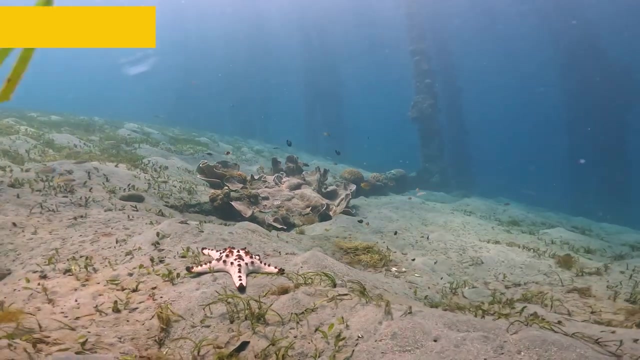 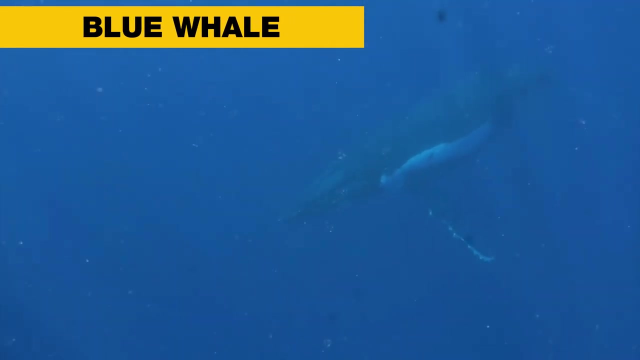 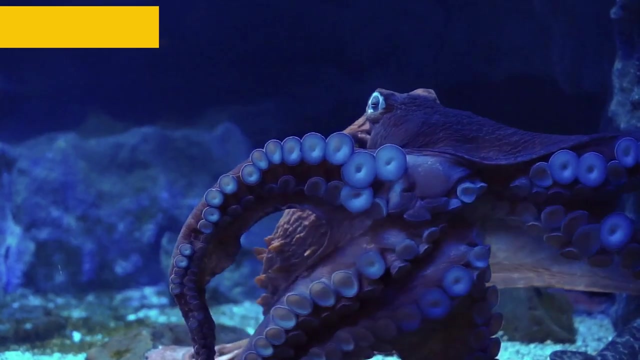 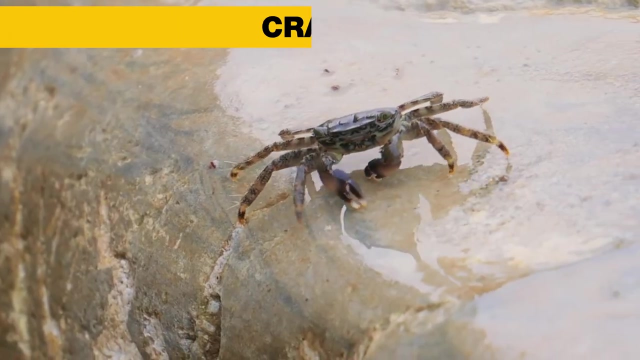 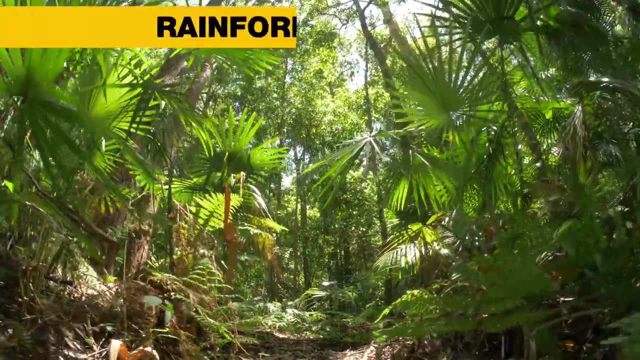 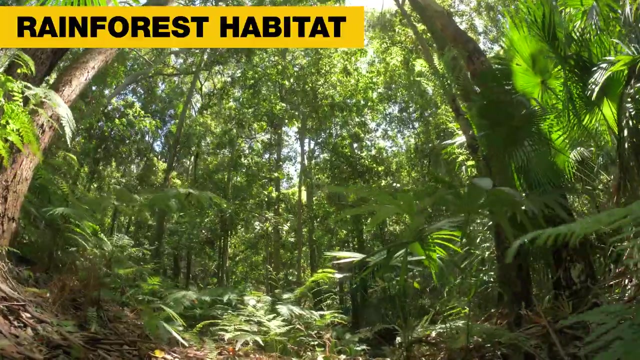 The marine habitat is the most biodiversity of all habitats. Here are some animals that live in marine habitats: Dolphin, Sea Turtle, Whale, Seahorse, Starfish, Blue Whale, Octopus, Crab. Rainforest Habitat. The rainforest habitat is a type of forest habitat that contains many trees and plants. 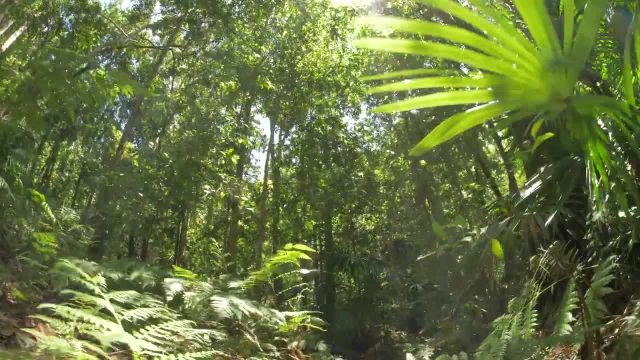 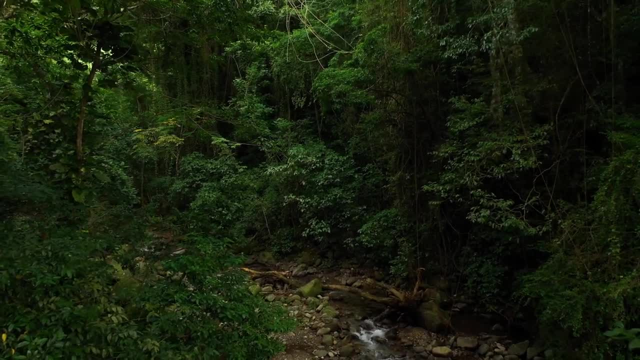 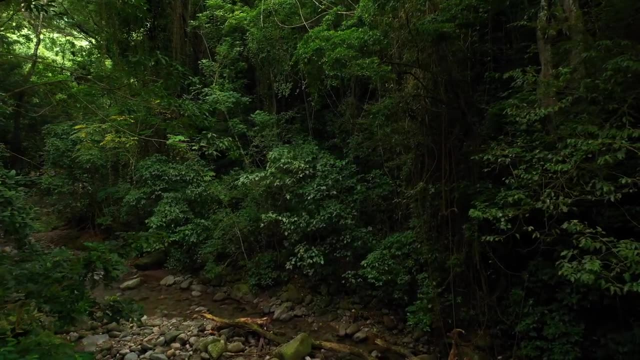 The reason it is called a rainforest is because of the high amount of rainfall it gets per year. The largest rainforest on Earth is in South America. The Amazon rainforest spans many countries, but is mostly found in Brazil. Rainforests are the oldest living ecosystems on Earth. 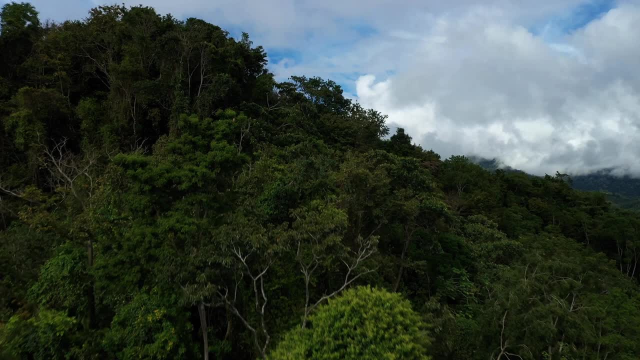 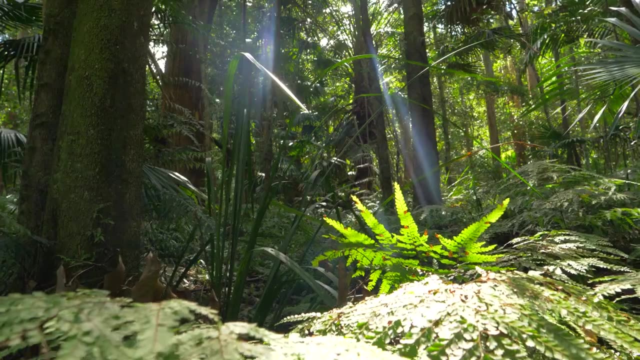 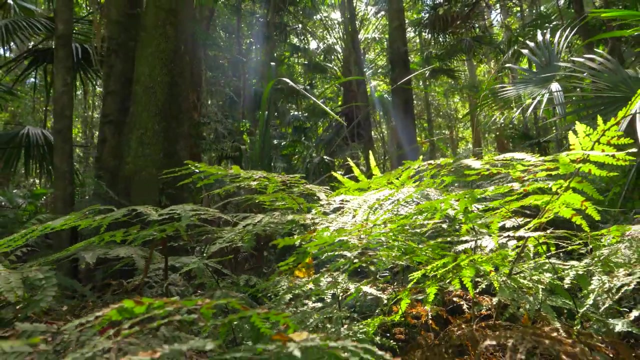 With some surviving in their present form for at least 70 million years. They are incredibly diverse and complex, Home to more than half of the world's plant and animal species, Even though they cover just 6% of Earth's surface. Here are some animals that live in rainforests: 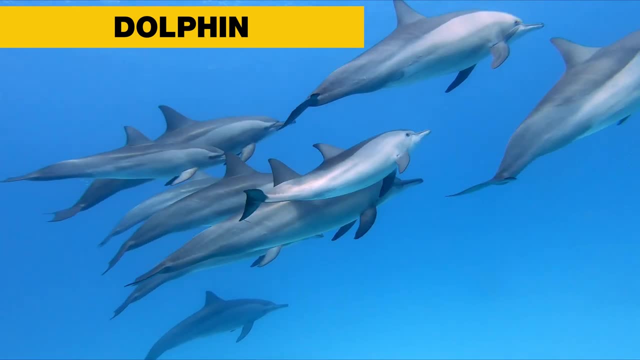 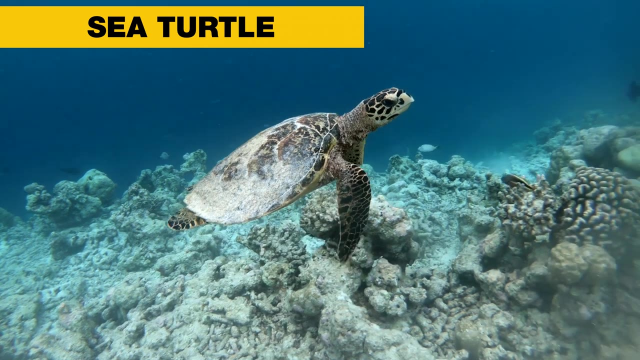 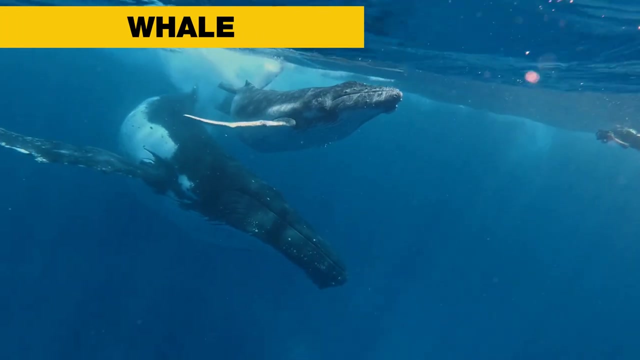 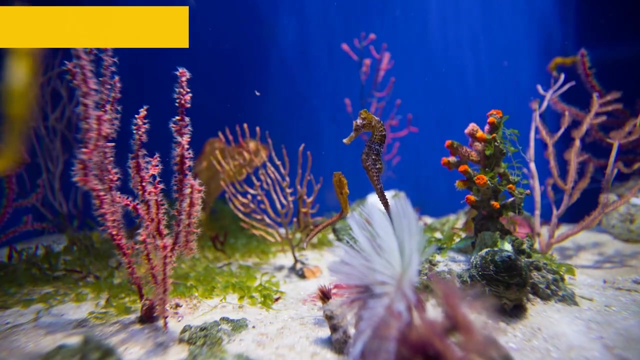 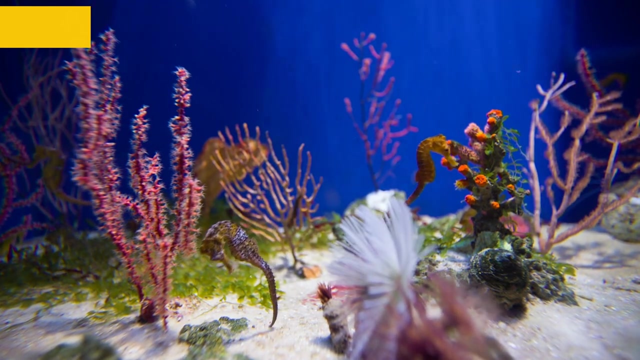 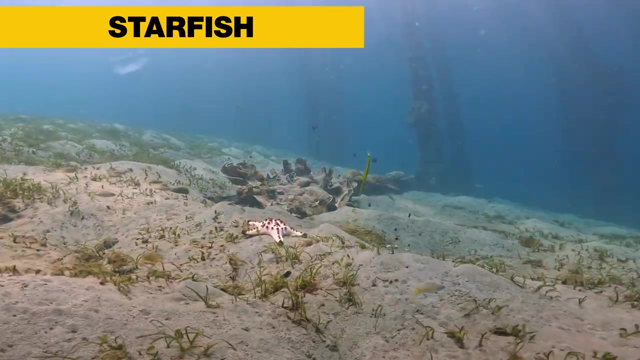 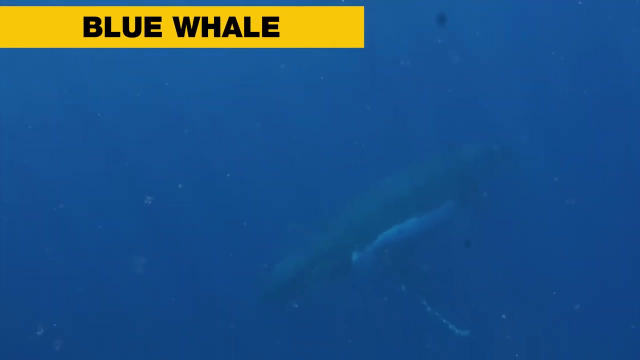 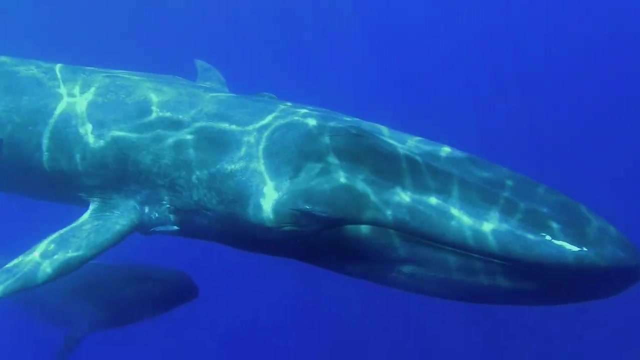 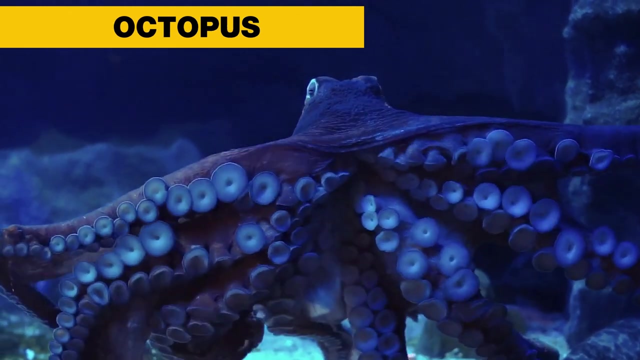 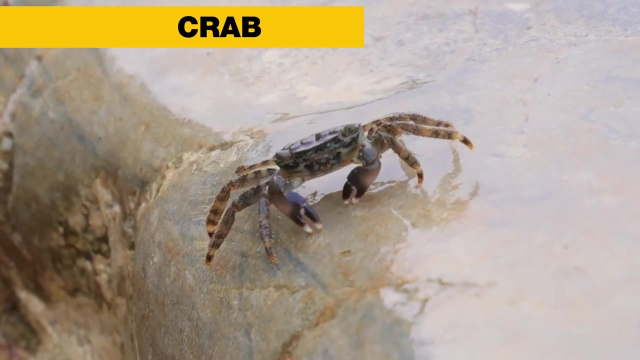 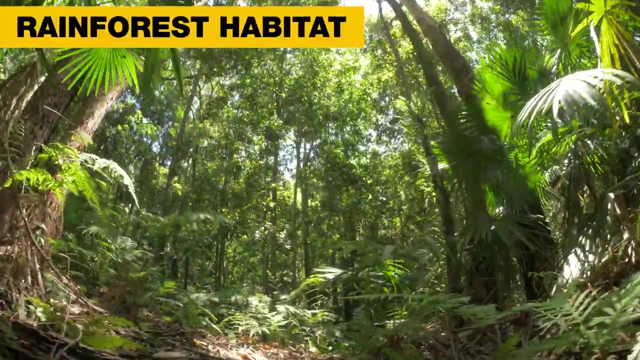 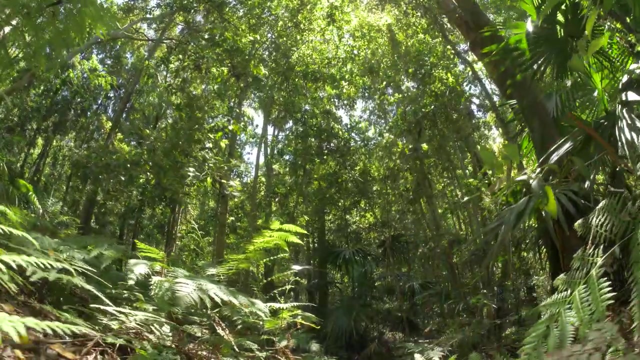 Dolphin Sea, Turtle Whale, Seahorse, Starfish, Blue Whale, Octopus, Crab. Rainforest Habitat. The rainforest habitat is a type of forest habitat that contains many trees and plants. The reason it is called a rainforest is because of the high amount of rainfall it gets per year. 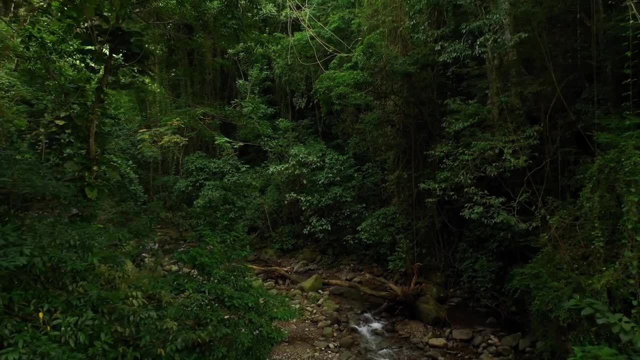 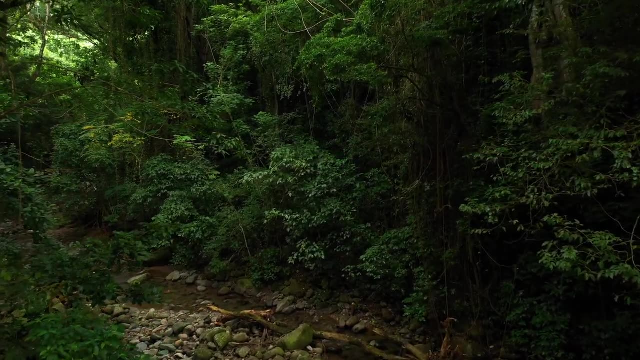 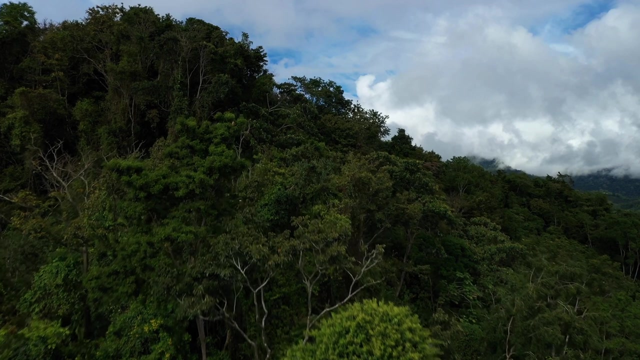 The largest rainforest on Earth is in South America. The Amazon rainforest spans many countries, but is mostly found in Brazil. Rainforests are the oldest living ecosystems on Earth, with some surviving in their present form for at least 70 million years. 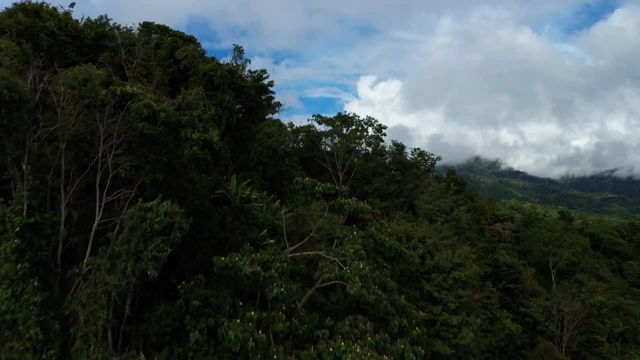 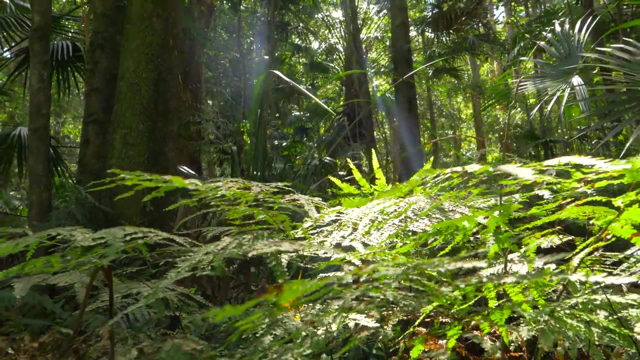 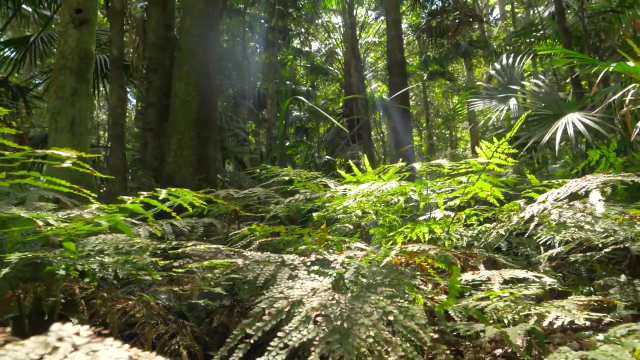 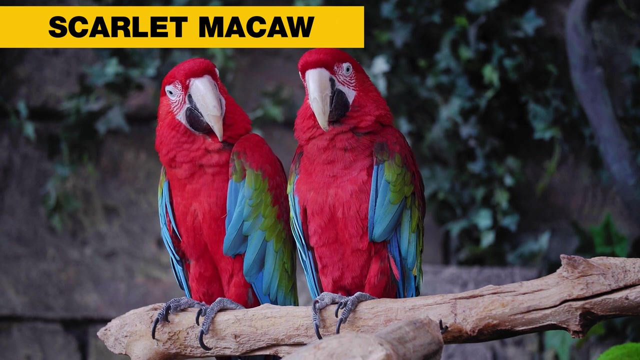 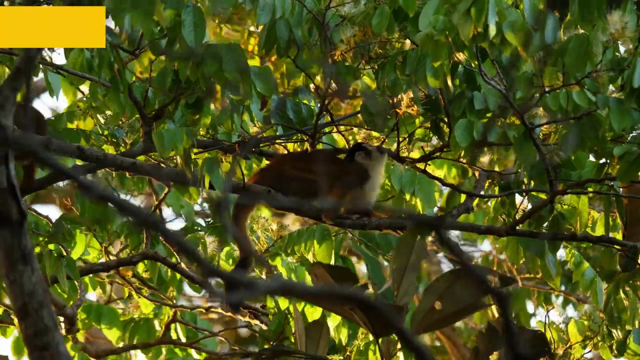 They are incredibly diverse and complex, home to more than half of the world's plant and animal species, even though they cover just 6% of Earth's surface. Here are some animals that live in rainforests: Scarlet Macaw, Holy Post, Bird Of Oath.